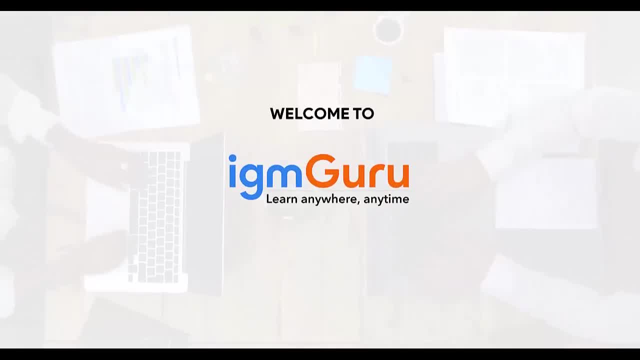 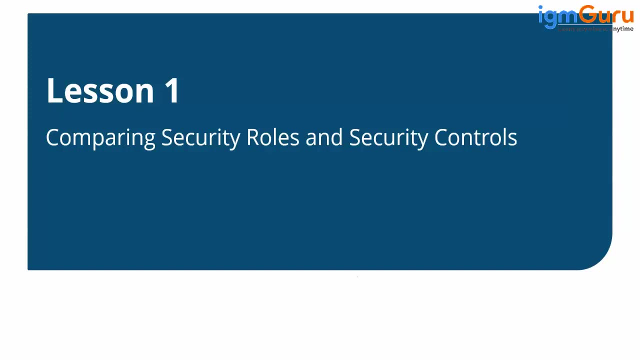 Welcome to IGM Guru. IGM Guru is one of the global leading online training and certification provider for IT expert by the skilled IT gurus to help them achieve their professional goals. Talking about the security, right? So, within security, what exactly we do See as a security professional, your work is basically to help organization to protect. protect against what? Protect against several types of attack, protect against the different type of issues normally organization is going to face there, right? So what are those issues? What are those attacks? That is what we have to understand in this security plus case. 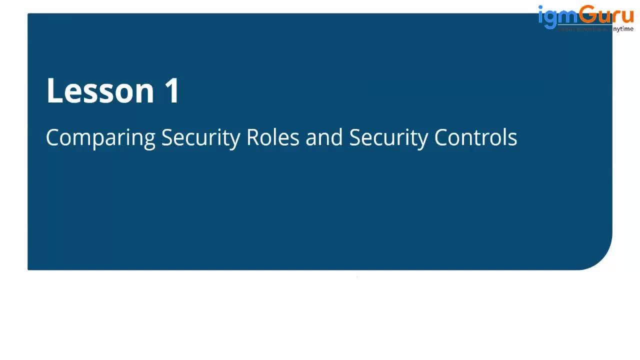 Curriculum and what are some of the protection control can be configured to improve the security right. So in the first lesson first we have a security role and security control. That is what exactly we'll discuss It means in this lesson. our aim is to establish the context for the security role and introduce the concept of security control, And there's lots of different frameworks also available. So framework basically going to offer you the structure and guideline. 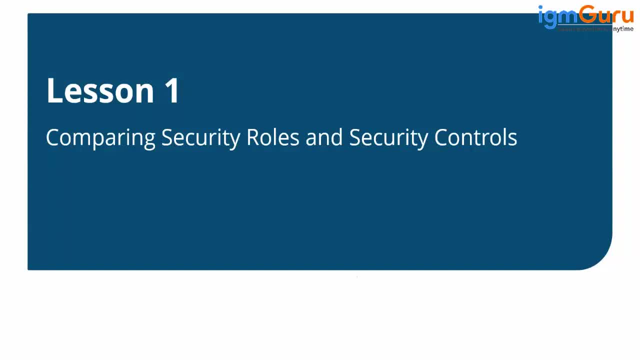 See, most of the time, whenever we are, whenever we are starting, we are not sure from where we should start. right, So that the structure and guideline will help you to at least move forward? Yeah, definitely, You have to make changes as part of the organization structure. 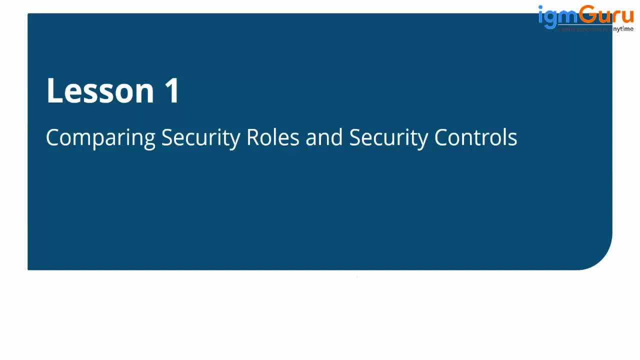 Every organization is having their own structure. They they always don't follow the strict guideline given there by the might be the government or and several other bodies there, But at least they will try to. Okay, Cover up all the requirement of the standardization body. 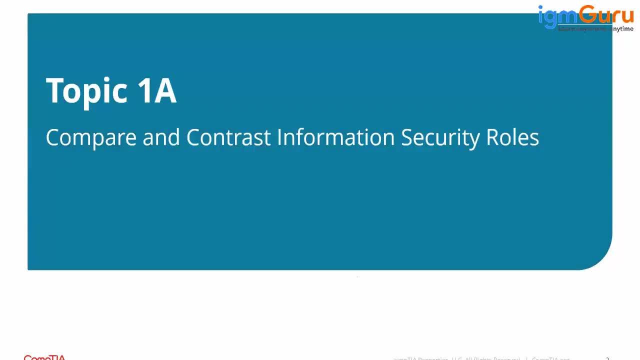 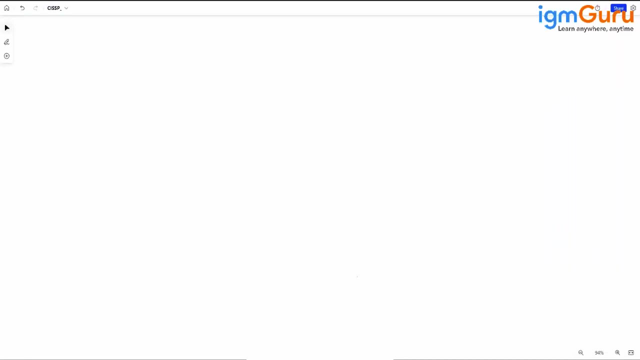 Right, So in this section we'll try to understand the same thing there. See, when we are talking about the security, One of the most important thing we have here is That we should know the context of the security itself. I mean from where we have to start. 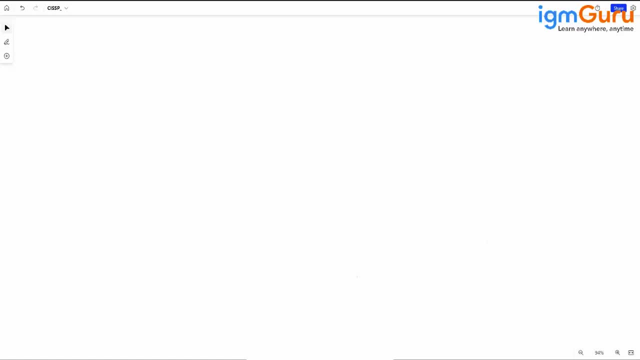 Right. So one of the most important point we have Is called the CIA triad Right. The CIA triad means see, at the end of the day, what we actually doing. We have several different type of Resources within an organization which we have to protect. And that is called as what asset. So you can simply say: anything which is valuable for the organization is called as asset. So valuable for what? valuable for the goal of the organization? The organization is going to set a certain goal That they are trying to achieve. 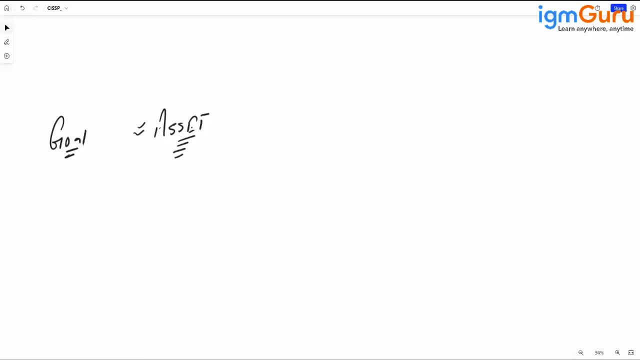 And to achieve that goal, they are going to have certain goals That they are trying to achieve, And to achieve that goal, they are going to have certain assets. Now that assets could be A very high end server. It could be unique infrastructure. 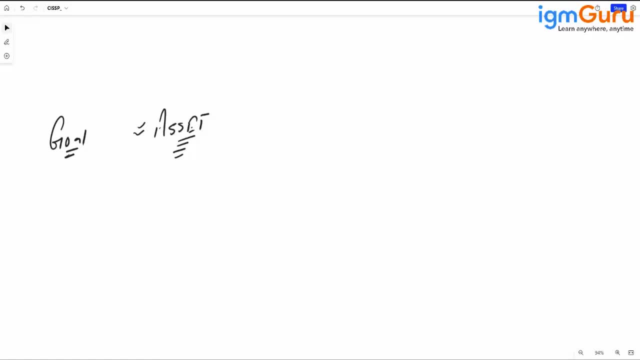 Like when we are, when we are dealing with petroleum, When we are dealing with gas stations. Right, We require a unique infrastructure. Right, That infrastructure is the asset for the organization. Without that infrastructure, they cannot do the business. Right, 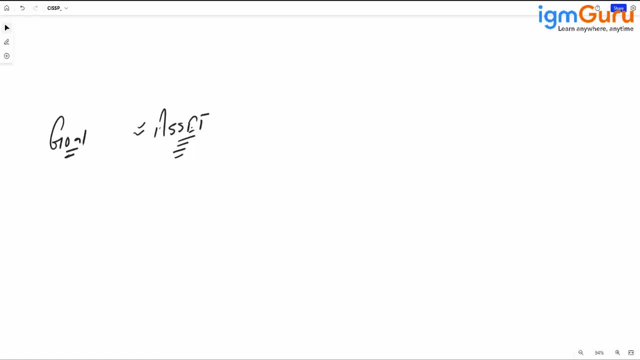 Similarly, To manage that infrastructure required some, You required some people, So that people is also your asset, Right. So anything which is valuable to achieve the goal of the organization is called as the asset for the organization, Right, And the problem is that. 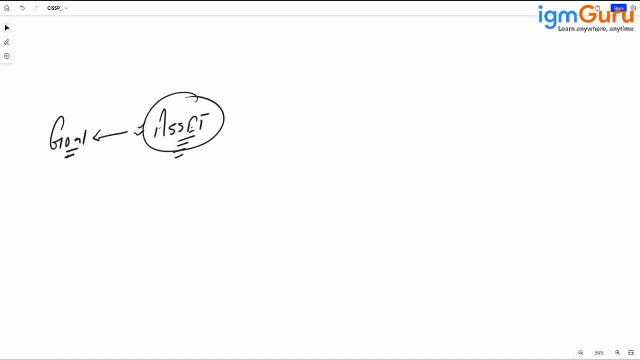 That is okay. See, if everything is good Is going well, There is no problem there, But problem is That there are lots of bad guys are also there on the internet, Right, Which is trying to take over that particular asset, Either for their own benefit. 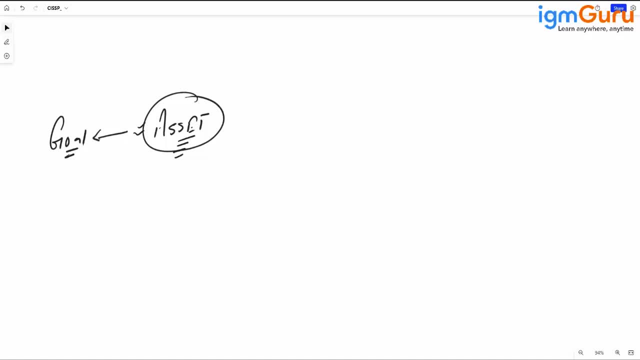 Or they are going to sell that particular resource to other, Another consumer. So So you will get some loss And whatever Right. So, In such case, what we have to understand, That every asset which we use to Take care or used to manage for our organization. 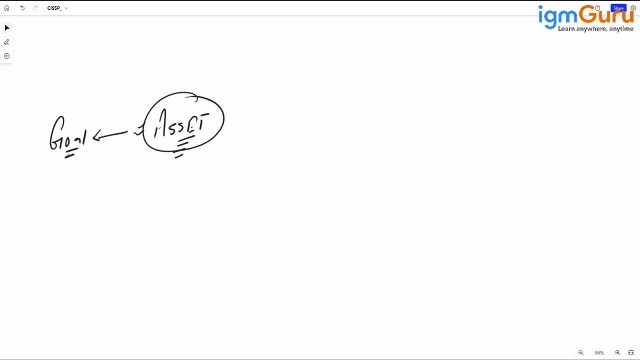 Right Is having certain set of loopholes. It There could be a No less severe Loophole, Could be a Very severe loophole, But there is some loophole Right Now. this loophole Is Simply call us. 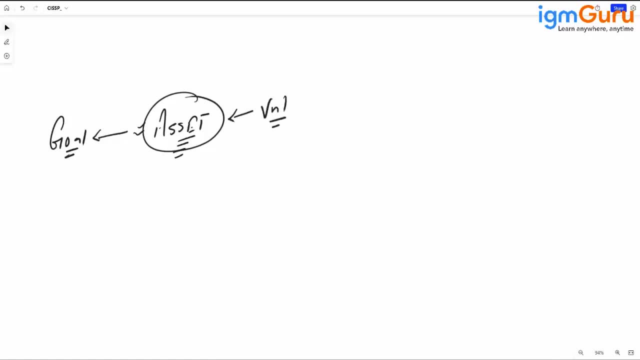 Vulnerability, Right, Right. So vulnerability is basically the loophole Which is possible Against your asset. Now, how severe that loophole? definitely we have to identify, But for now we need to understand that Not all the resources Is equally secure. 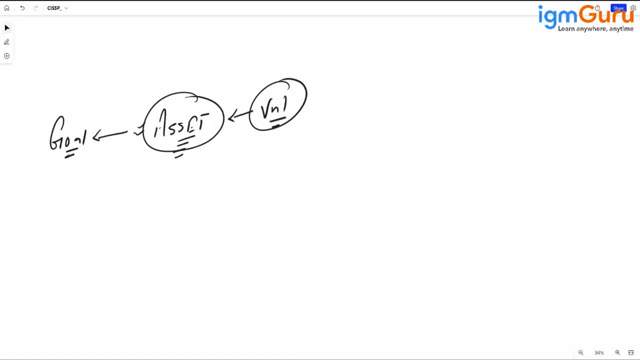 Some are having less severe loophole. Some are having Very Severe loophole Right. In such case, We have to understand those vulnerability, Because if you don't know what is that vulnerability, we cannot go for the protection as well. The problem is that 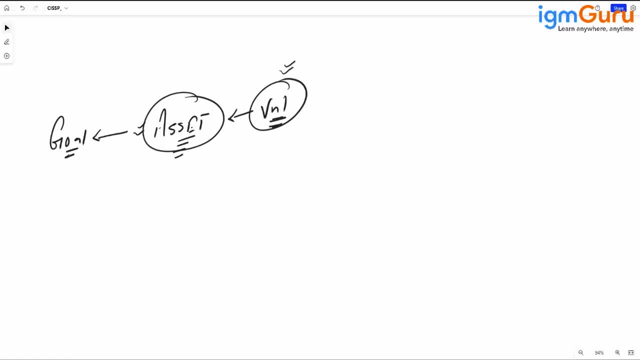 Even if this vulnerability is there, there is no any problem. Problem is there because there is a threat available around the internet Which can take benefit of this vulnerability Right. So there is a vulnerability, There is a loophole. So far There is no any problem. 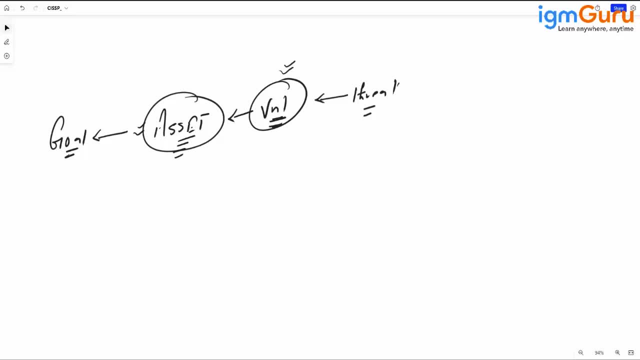 But let's suppose there is a threat created to exploit this vulnerability. Or you can say There is a threat created to take benefit of this vulnerability. The problem will going to arise there. So if this threat, We'll try to take over the vulnerability. 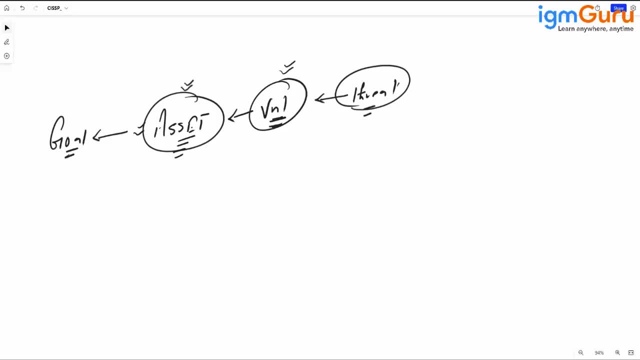 Then in such case, they can Control your asset very easily. Let's take an example: in your home There is no need door Right And there is no need or lock. In such case, what will happen? The intruders can take benefit of that vulnerability and they can. 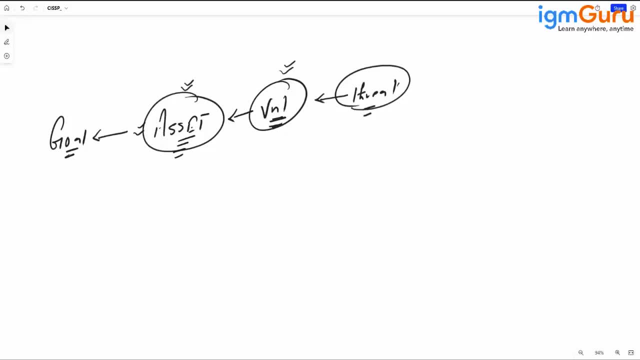 You know, do some damage. Correct, Right. So that is one simple example of this threat. Another one: So let's suppose there is no need threaten. I think you live in Canada, Correct? Yes, Let's suppose there is no need threat in Canada. 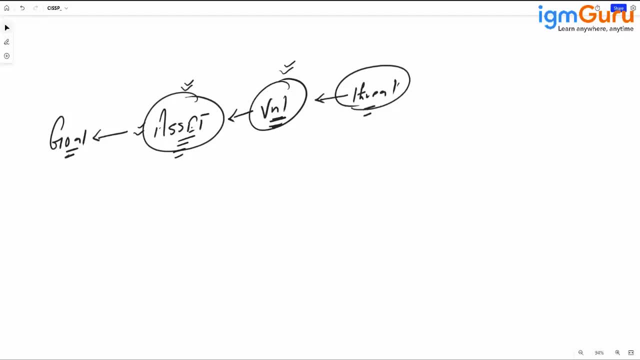 There is no need tapes available. There's only looters available, Correct. In such case, even if there is any vulnerability, There is no an issue for us. Correct, Right Problem will come when these both things are actually comes together. 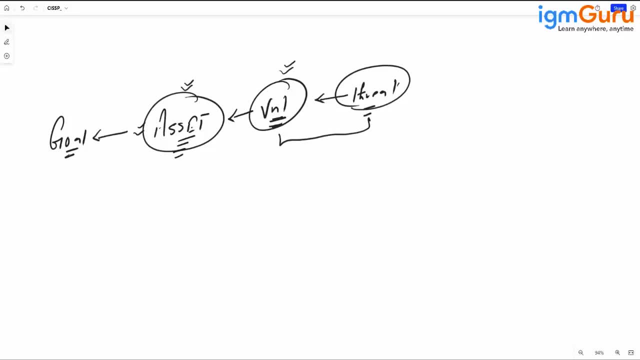 It means there is a vulnerability and if there is an associated threat also available And because of that There is a risk Present on your Asset Right. So on. as a very simple note, if I need to define risk, risk is the possibility. 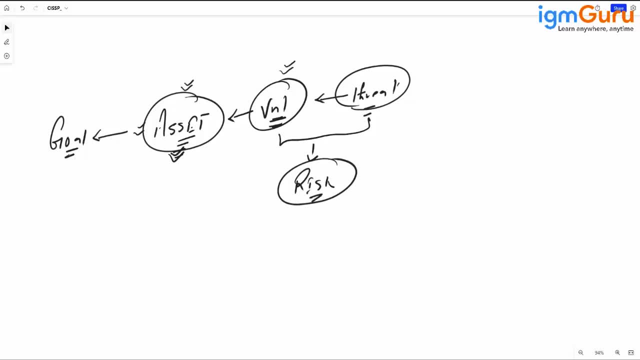 Of a certain event Giving some negative Issues, Right, So possibility of an event and their negative consequences, that is called as risk. So possibility of an event like a wireless attack- Wireless attack on your system can possible, Right, So that's a, it's an event. 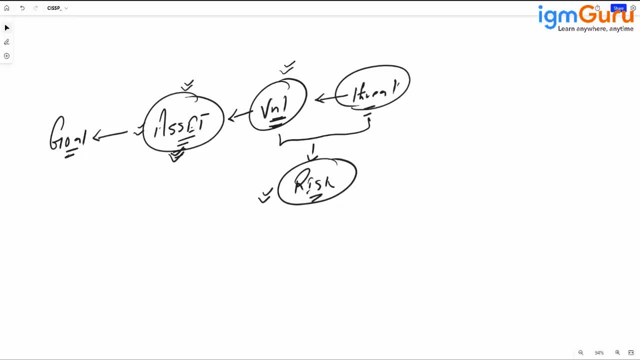 Wireless attack is an event, But because of that virus attack, if your file got corrupted. That is the consequences, Consequences, Right. So if both comes together, then only there is a risk on your system Or in your organization, Correct? 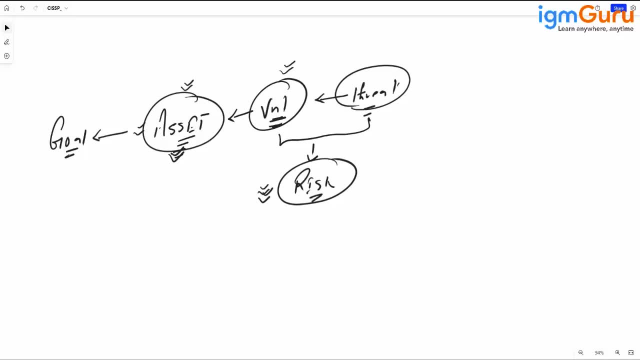 Right. So organization first will try to understand what are the risks available And then after they will go for the fixes. Right Now the question is: let's suppose I know there is a threat available, I know there is a vulnerability available. 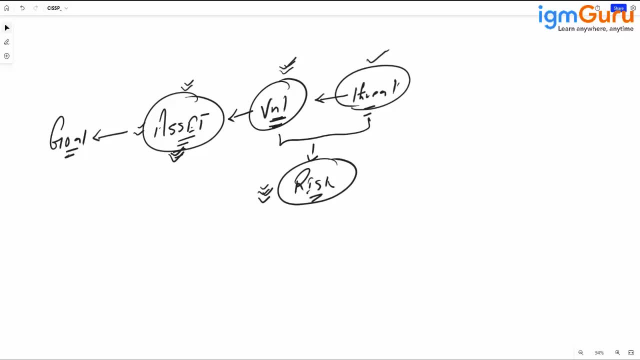 Then what Then? what we have to do Then. in such case, you have to understand, or do you have to measure, What key pillar of security These two are basically breaching. Now remember, whenever we are trying to measure security. 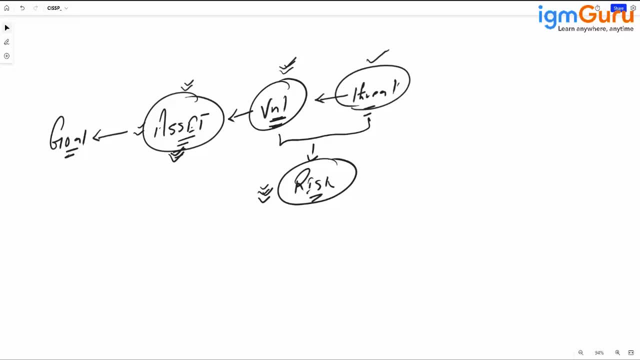 Okay, Instower asset. We simply check What exactly this asset require. So remember: not all every organization is having equal priority, Right? If you go and talk to a military organization, they have a different priority. If you don't go and talk to the government organization, they have different priorities. 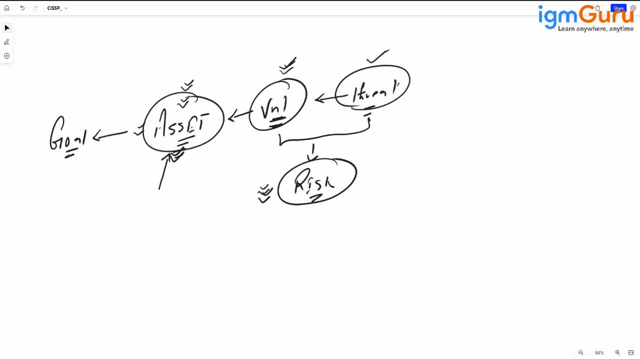 And if you talk to the government organization, they have different priorities, Right? If you go and talk to the organization? If you go and talk to the organization, They have completely different priority. If you go and talk to the organization, They have different priority. 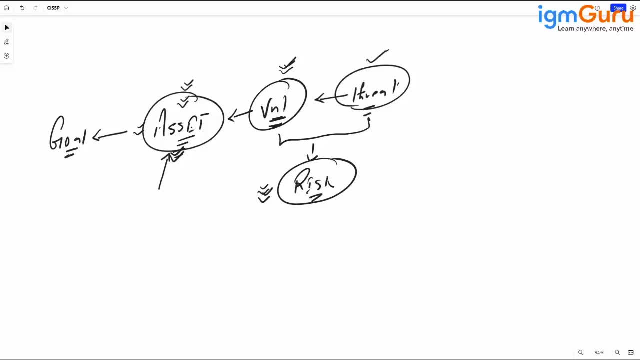 Right. If you go and talk to the organization, They have completely different priority, Right? So every organization is having their own priority. Accordingly, the assets they are going to purchase on, accordingly They will try to make the business. So, whenever we evaluate, 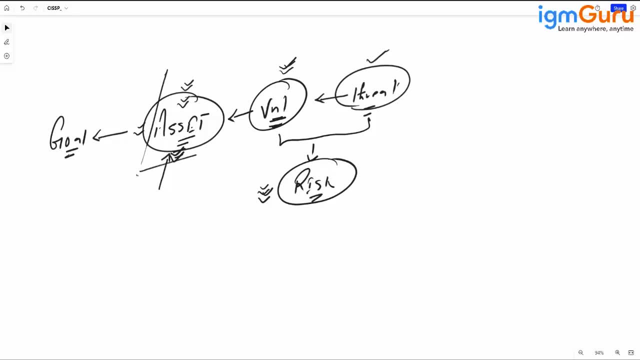 Security. We have Key pillars to evaluate the security. The first key pillar is confidentiality. So confidentiality means making our information confidential, only available to the people who is entitled to access. So information should be known to a certain group of people only who is authorized to access it. 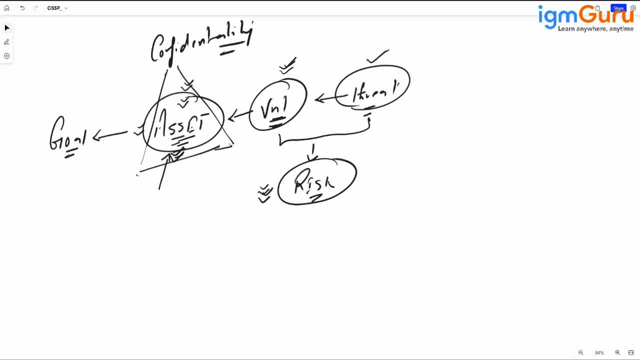 So if I am trying to maintain security for my asset, I have to check how much confidentiality we require for that asset. Right, So that one we have to check. Secondly, there is a possibility that integrity can be also breached. Integrity breach means the information can be changed without your. 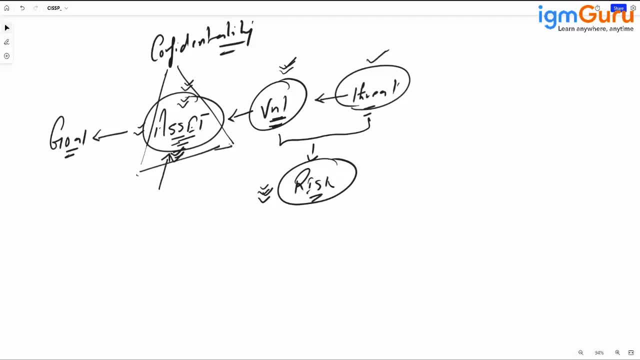 knowledge. So if the information is changed without your knowledge, then also it's a damage condition because based on this change information you cannot do the business correct Right. So this is called as the integrity. So integrity is another key pillar which ensure that your system or resource remain same. 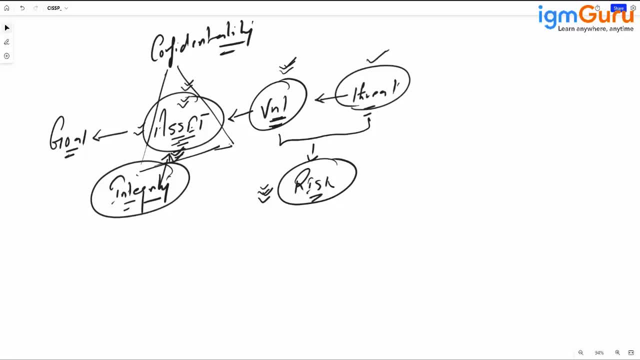 until unless it is changed by the authorized user. It means only authorized changes are acceptable over the asset, Unauthorized changes, whether it is from authorized user or unauthorized user, both are not acceptable. So integrity will maintain and ensure that your information will be only changed from the authorized user. It should not be changed from the unauthorized user. 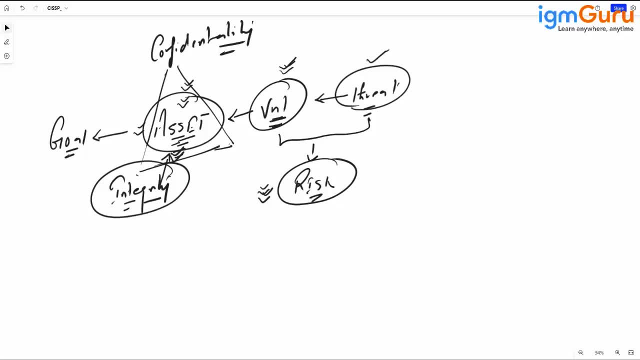 And if there is any change, we should be able to detect that because based on that change information, if you are doing any processing, there is a complete chance that your system or your organization will face a huge damage. Let's suppose I am managing HR operations. 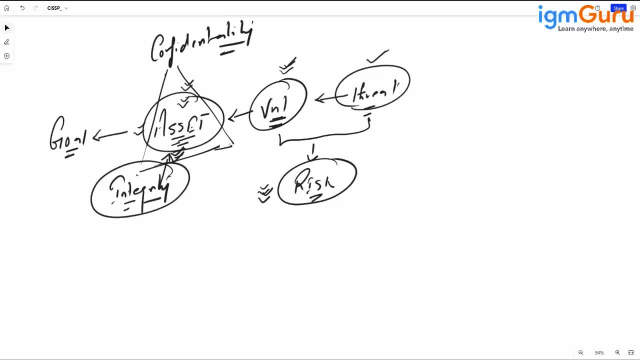 where might be. today I need to disperse the salary of my employees. In such case, let's suppose the salary seat has changed without my knowledge. right It means whatever the dispersal will I will do. that is going to be based on the change information. 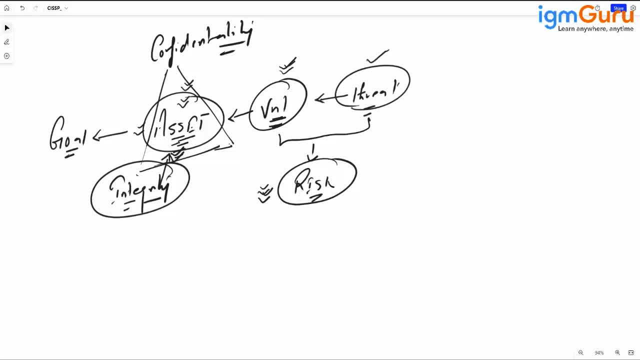 So we should have a way through which we can detect such changes. Otherwise, this will create a devastating effect on the organization Right. So this is another key pillar of the system. The third key pillar of the security is availability Right. You cannot only focus. 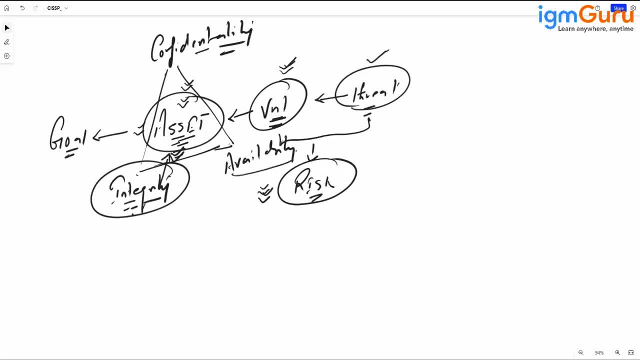 on the confidentiality and integrity. you have to also focus on the availability. If the information is not available to the customer, how they will do the transaction right Right? Sometime we focus more on the confidentiality and because of that, availability is going to suffer. 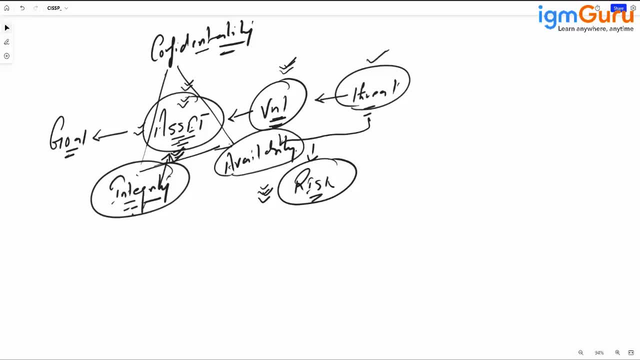 Let's suppose you had. you had taken lots of precautions, lots of measures, and the asset which trying to protect is under your control. That is okay. But whenever you're trying to access it, there is lots of delay happening. Let's suppose you have to. you have to unlock three or four. 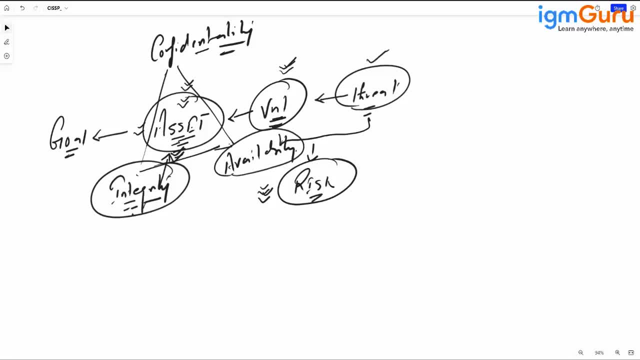 locks there. Okay, And might be. there's lots of protection. you have to turn off and then only you can access your asset which is present in your home right. It's going to create a kind of delay which will impact your availability. See, customer will be not be going to happy. 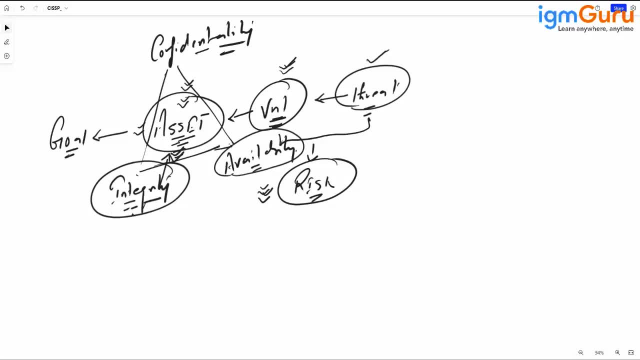 if they are trying to access the information and the time And the moment the information is available to them is having us very huge delay, right? So this is going to impact the availability and in such case they will try to move into another location. Let's suppose I'm trying to. 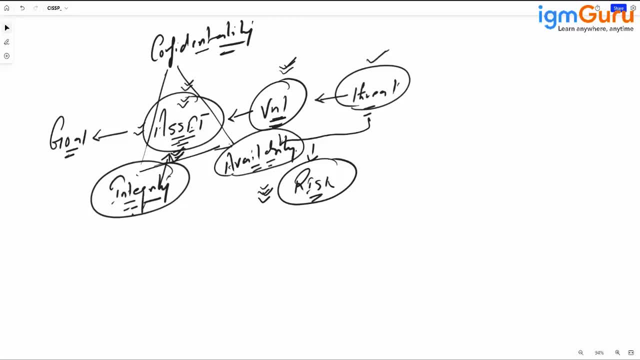 do a shopping today and I went to Amazon website. They're a. their website is down today because of any reason. right, I tried one time. I tried two time because Amazon was was my favorite. i tried even the third time as well, but because after third time i lose my. 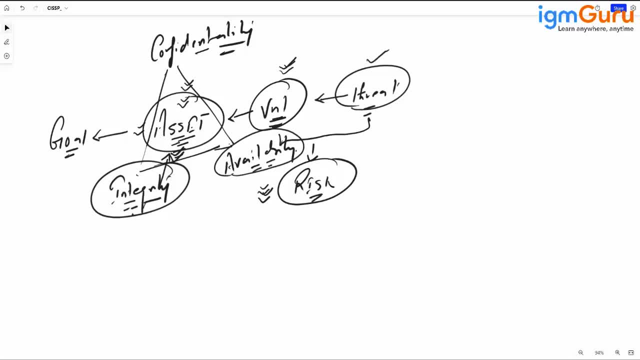 patience and i move to another website because i, at the end of the day, i require a product, but then i'm coming getting from amazon. might be flipkart or any other website, that doesn't matter for me, right, i all, i require the resource. but what is happening there? amazon is suffering here. 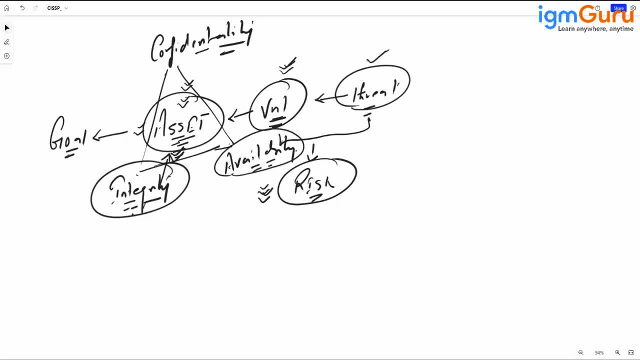 why? because of the- might be some, some in, yeah- huge protection they had configured. because of that users are not able to access, or might be their server is down today. it could be any reason, right, but at the end of the day, availability is also important for the business. 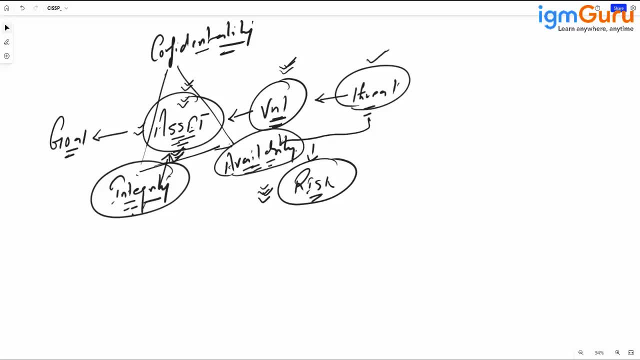 and availability can be suffered because of n number of reasons, like: let's suppose you have one single system and today it is having some problem. it is not booting up right. then you are not able to join the session right, so it is going to impact the availability. 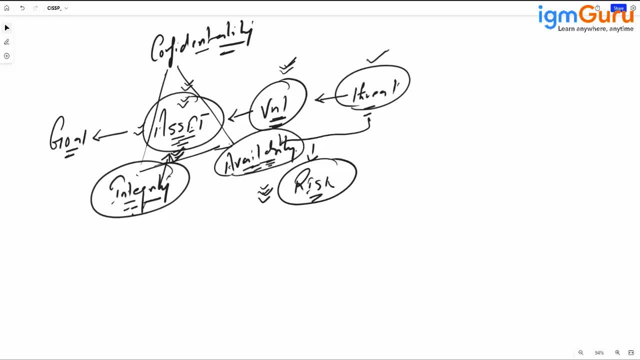 right. similarly, if you have single hard disk to store the data, if that hard disk is down, then you are not able to fetch or store any data on the hard disk, right? so that is again impacting the availability. so availability is basically getting suffered here because of n number of reasons we have to 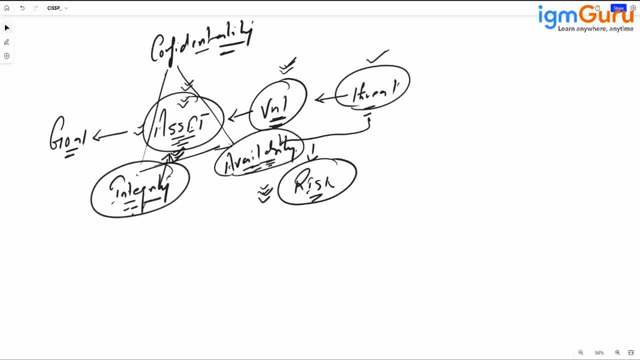 ensure that all things is implemented properly, right? so whenever we measure security against the asset, we always take care of these three key pillars: confidentiality, integrity and availability. right, that is making sense, yes, cool. so if security is there, now there is one more key point. so sometime, what will? 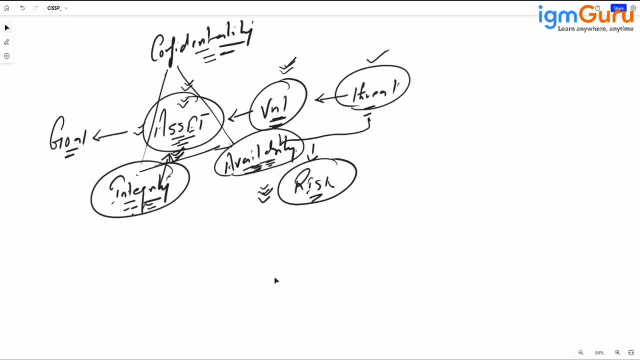 happen: a certain attacker or certain user had done some action and after that they are actually denying, then no, i have not done this. actually, they are thinking까r. it was custom action, right? so this is called the repudiation attack, right? so repudiation is. subject: is denying. 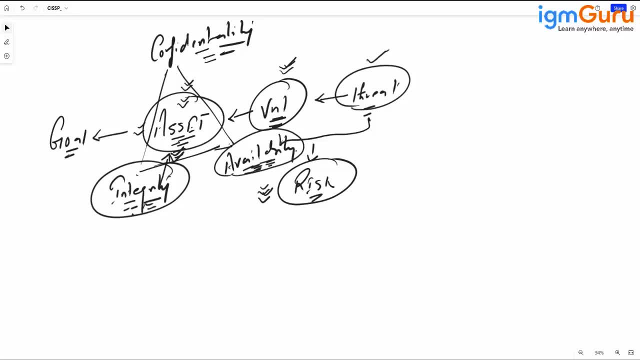 from their action what they had committed. why it is happening? because you don't have any mechanism through which you can detect such activity. let's suppose i'm doing some activity and it is getting recorded. i cannot deny from my actions why. because there is a log, there is a proper recording. 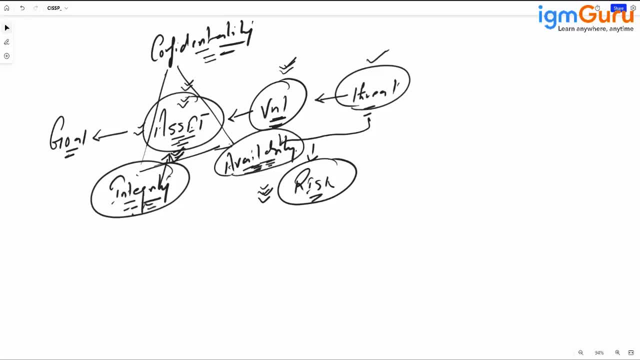 available, right? so that audit, so that is called the auditing. so with the help of auditing you can, you can actually prove that whatever committed is basically true and that is committed by a certain person. right? so this principle is called non-repudiation, right? so non-repudiation where 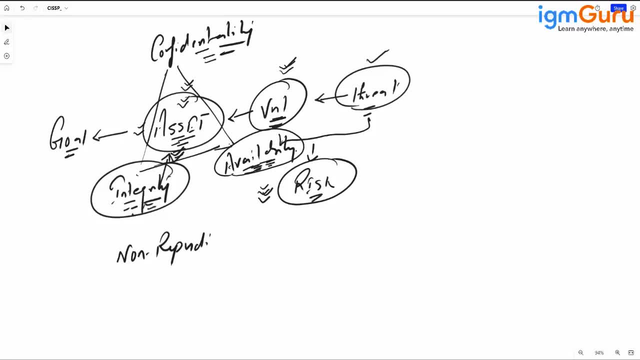 subject cannot deny from whatever action they had committed. so non-reputation is what is one of the control available against what against you know, against what you know, a repudiation attack. so, uh, okay, now for that. your non-repudiation is all about enabling the audit. 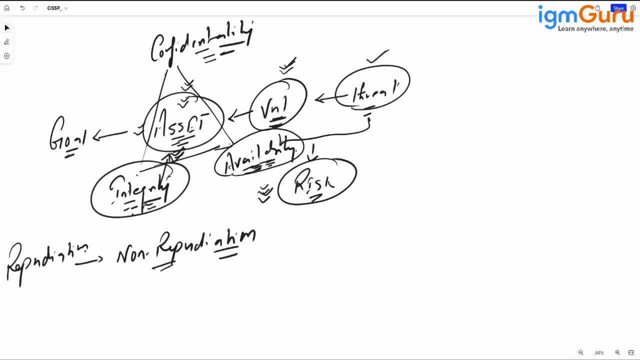 log to ensure that all the activity happening from the user site that is getting recorded. so that is another very important point here. now remember, whenever we are- so now we know that- how exactly we need to talk about the security. i mean, what are the key pillars we have to check? 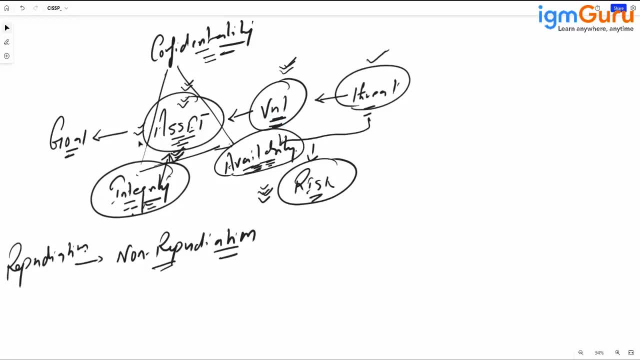 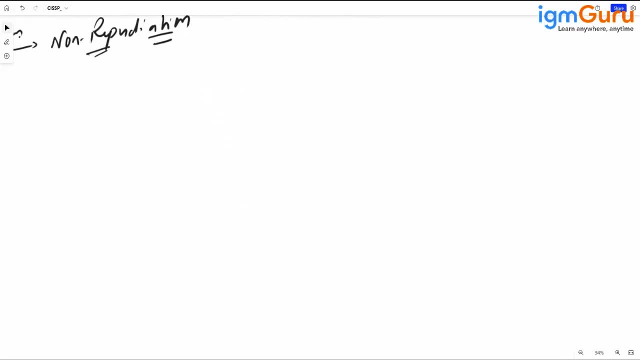 what is risk, what is vulnerability, what is threat? so i hope this is clear. yes, good then. another thing is that whenever we are talking about the security control, how exactly we should start with. i mean, let's suppose you are working as a security engineer, you have to implement the control, so how? 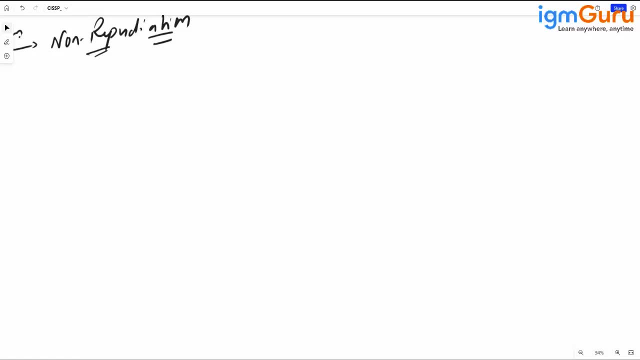 exactly we should start with. as i told that, you know we generally follow some certain structure, some some framework. so framework will provide you a different uh, overall defense architecture which will help you to guide how exactly you should have to move forward. what we have to understand: there are multiple different type of threats available around us. previously, we were 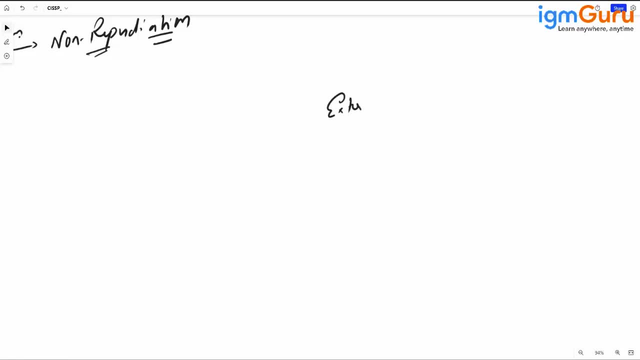 so much focusing on the external threat only. it means anything which is coming from outside. that is a threat for me, right? but nowadays that is not the case. nowadays, even the internal threat is also there, and there was a case study where it was still told that most of the attack is coming because of the internal reason. it could be. 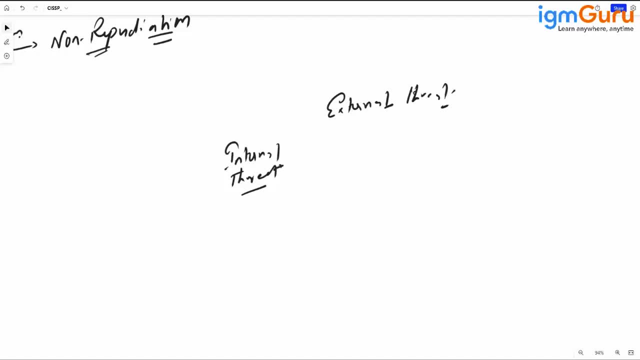 intentional, it could be unintentional, but it is because internal users are not aware about the security issues most of the time the breaches are happening okay. so we have to first understand that, why a particular threat can realize against your organization. that is the most important. and then 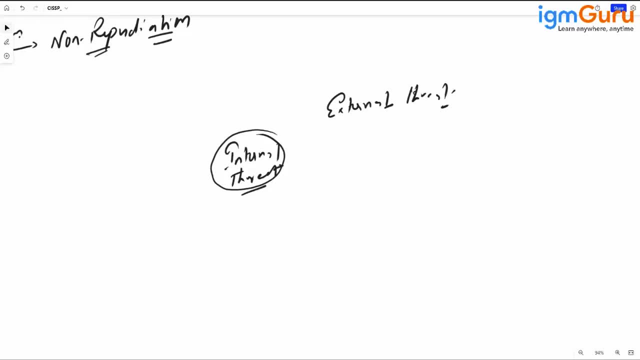 based on that, we can actually go for the implementation of control, the controls, like i mean first we have to identify what is the threat. right, then we need to accordingly move forward, right. so identify, then- i mean first you have to identify what exactly you are trying to protect, i mean the asset. 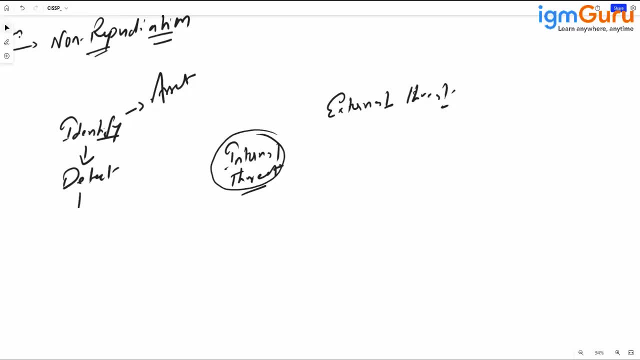 right then we have to detect the threats, right then, if the detection is done, we have to respond to that threat. right? and let's suppose that if there is any damage done during the compromise, then we have to also go for the recovery action, right? so remember a framework. 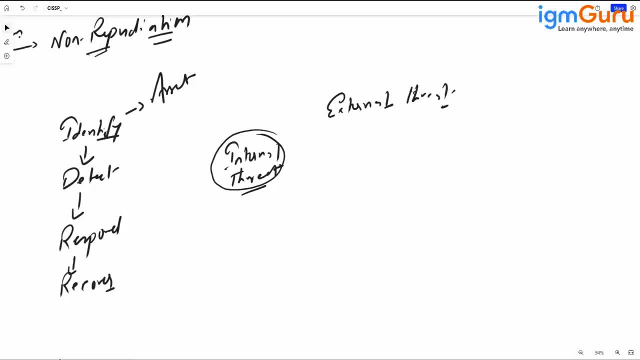 will simply going to provide you a kind of a structure, but that structure could be totally different from the structure to structure. it means different structure is actually having their own way of defining how the things will actually move forward. right, and so the other thing we have to do is, from the information security competency side. 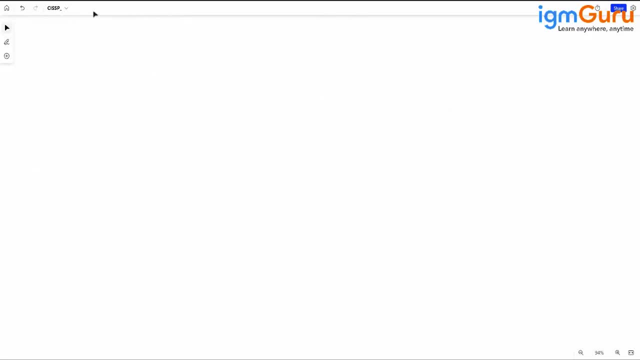 some of the most important activity which we have to do. like, let's suppose there is a asset which we are trying to protect, first you have to do is call the risk assessment. so risk assessment is what we need to know. what are our vulnerabilities and, yes, what are the. 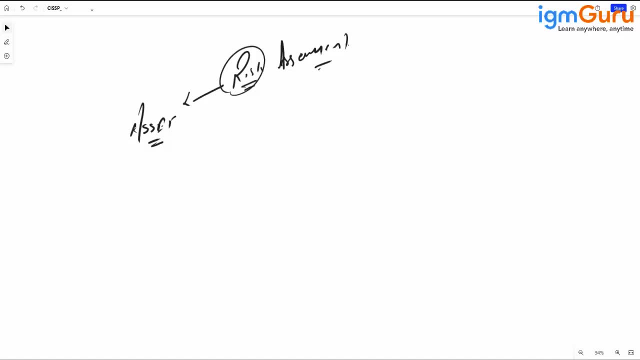 threat. so that is basically helping you to understand the risk. remember risk is the on a simple known. if I need to define the equation of the risk, so risk is the combination of threat, vulnerability and impact and impact concept, right, consequences, correct. it means whenever you are trying to do the 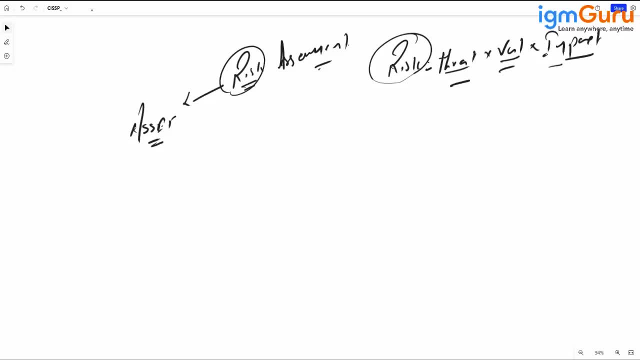 risk assessment. we will try to evaluate these all thing and based on that we can actually decide whether the risk is high or low and accordingly we have to take action. then we have to understand what are the threat actor. so threat actor means a person who is getting benefited because of this. what attack? or because 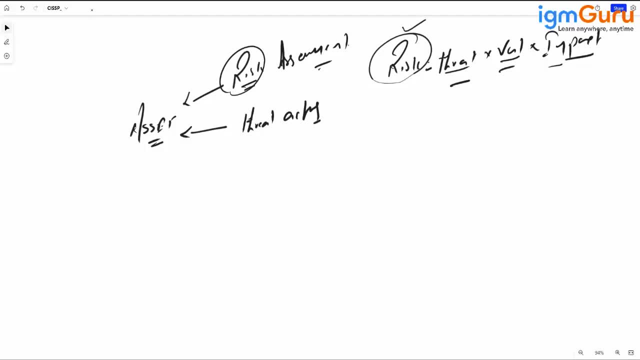 of this risk over and, all right, it could be your competitor. it could be just a script kitty guy who just learned those were security and they'd wanted to just do the attack. so it could be a number of person, but anyone who is getting benefited because of that act is basically. 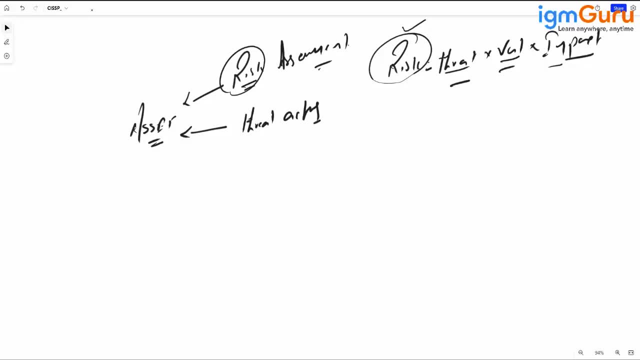 called as a threat actor right what we have to understand? that we know that such threat or threat actors are there and accordingly we have to put the access control. access control means only privileged users are able to access my resources. unauthorized users should not be. but sometime there may be a. 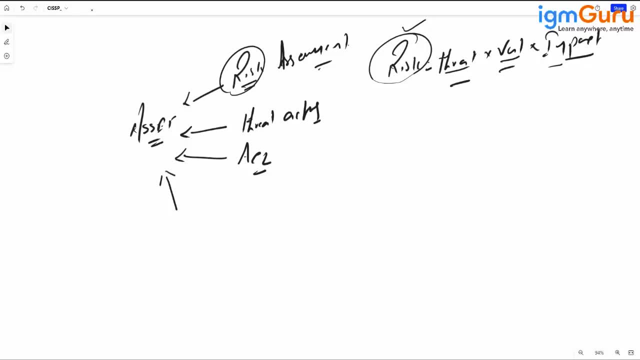 possibility that the unauthorized user will try to access your information. in such case we have to ensure a proper audit is happening against that right. and then we have to put the access control and then we have to ensure a proper audit is happening against that resource. it means whenever someone is accessing the resource there is a 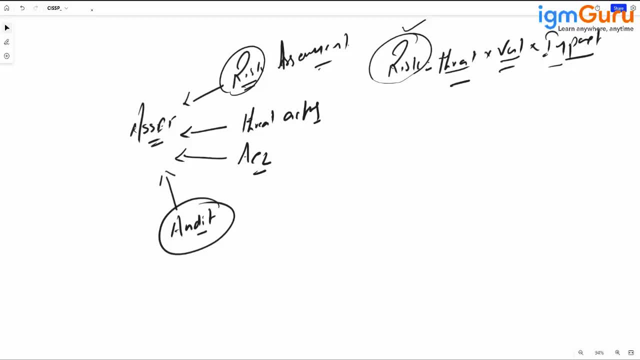 proper log it generated, and that lag log will help you understand whether a certain resource is accessed by only the authorized user by, or some unauthorized user is also trying to access my resources. right, but if some unauthorized user is trying to access your resources, this is basically a kind of incident for 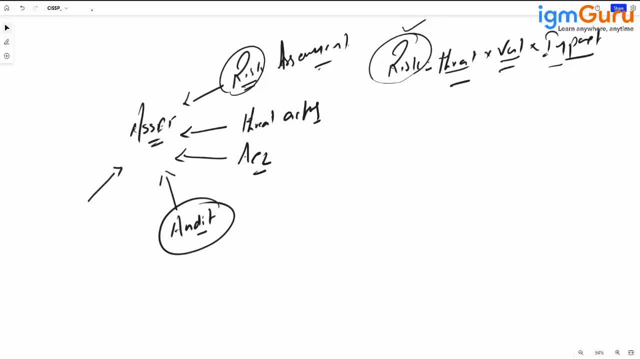 your organization, right. so incident is what. any we event which is negatively compromising your confidentiality, integrity and availability, that is called incident, right so again, repeating: any event which is negatively compromising your CIA is incident. so in such case we have to have some incident reporting and response procedure. it means someone have to report. 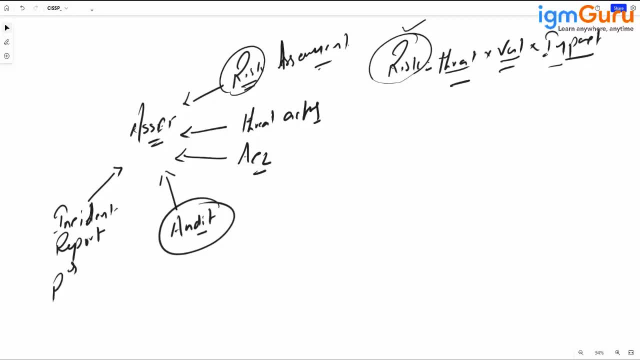 that such incident happened and accordingly the response should have been given- see the main agenda of the incident reporting and responses. to ensure that quick and calm response against any risk, so the negative or any issues can be reduced very easily. we also have to do the business continuity planning, BCP. 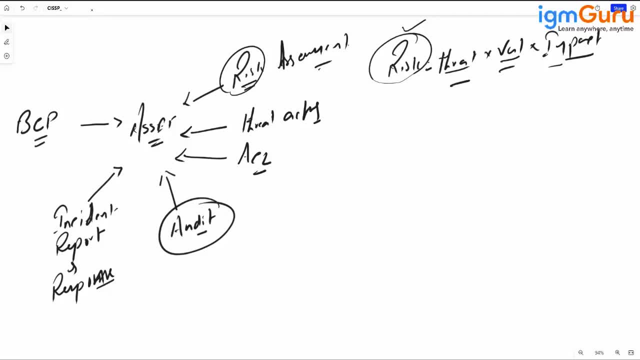 see there is a might. there might be possibility that attacker sometime is succeeded in the incident. if you are able to respond on time, that is okay. but if you are not able to respond on time, in such case you are in a disaster mode. your information is compromised. they had 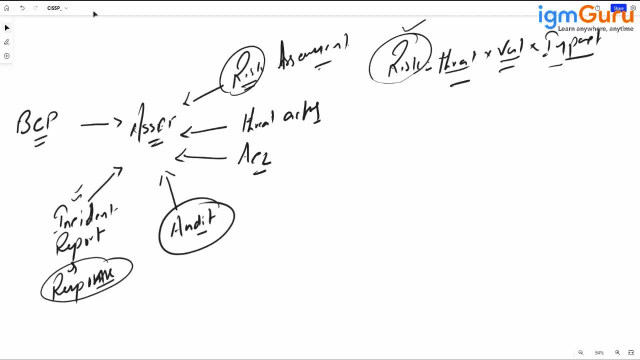 already downloaded and now you are in a disaster mode. let's suppose your sensitive information is accessed by the attacker. what they can do, they can publish on the internet, right, they can ask you for the money, whatever could go ahead and number of reason. so now you are in a disaster mode. and if it is in 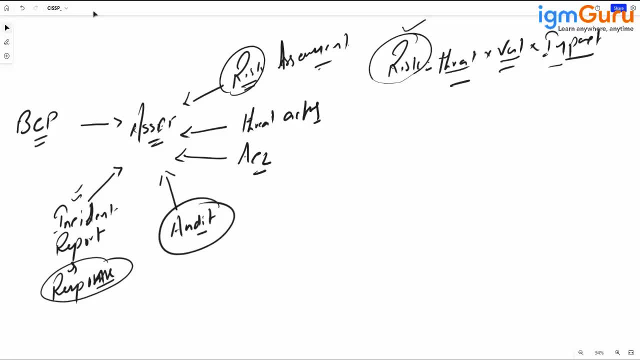 a disaster or may not disaster mode. it means now is a time to ensure that we can provide some response and maintain the business continuity. because of disaster, there could be a business downtime. let's suppose there is a natural disaster and because of like hurricane or land escaping right and because of that your entire business is down right. in such case, 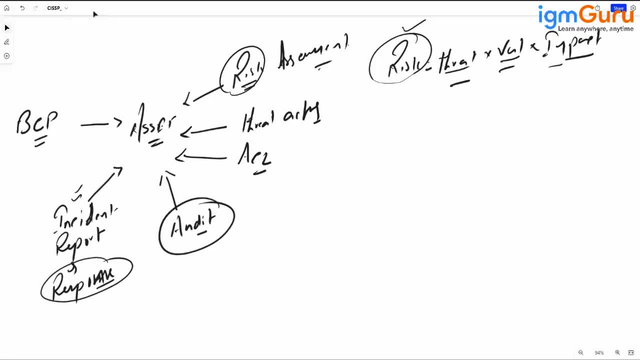 you should have a plan. so if such incident happened, then we should have a plan so we can at least maintain the continuity of the business from it might be from the another location, right? so I have a question here. right, location wise, I understand BCP, but if it is like, say, for example, they are attacking our asset, is? 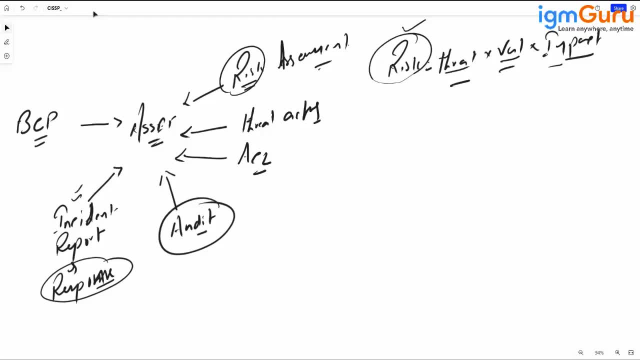 not like infrastructure, maybe it's. it could be like information. how do we create BCPs in that situation then? in such case, we have the backup option right. nowadays we have multiple option. we can take a backup of the data. we can take the backup of the entire. 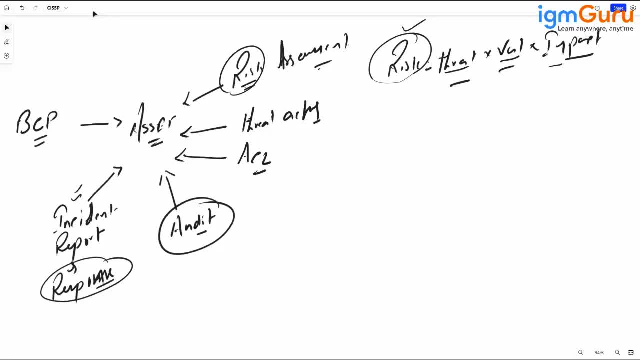 server. we can put it on to the cloud and we can run it from the cloud in the meantime. so when we are recovered fully, then we can move back to our on-prem infrastructure right. so in case of information, we have a backup procedure. we have multiple disk available, so even one of the disk is 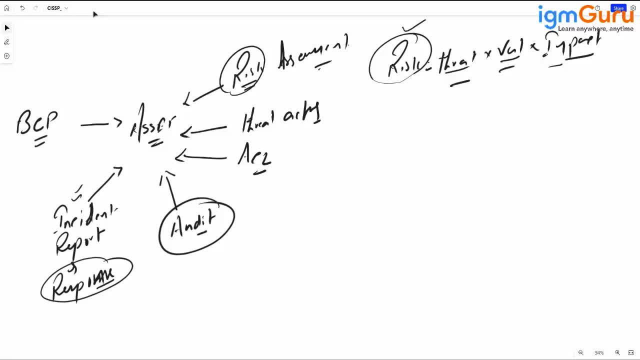 down, we can still maintain the continuity right. so BCP is another plan and the most important thing, that whatever you are implementing right, it could not be fruitful if the users are not aware about how to implement that. it means we have to have the security training as well. training and education. 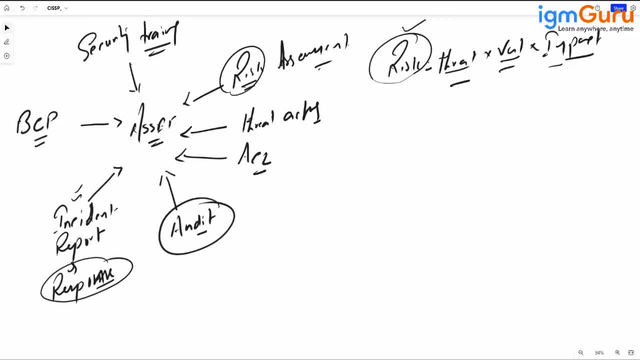 is very much important because, without that, users may not able to do the things which you, which you actually want in your organization, to implement. now the question is: who is responsible for this entire activity and who is responsible for the? remember, multiple different roles are there. who's responsible for that? at the end of the day? 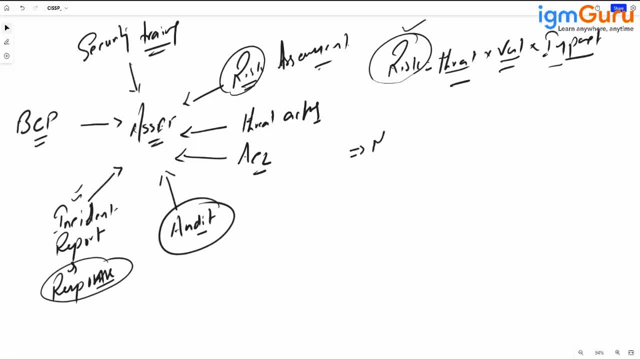 accountability belongs to the management right, so it is the management who is accountable for protecting the organization. ceo cto, co. these are basically the roles. who is responsible for ensuring that your organization is continue to operate and you know, in the front line of in the might be in the market right, but definitely to provide security, they will be giving responsibility. 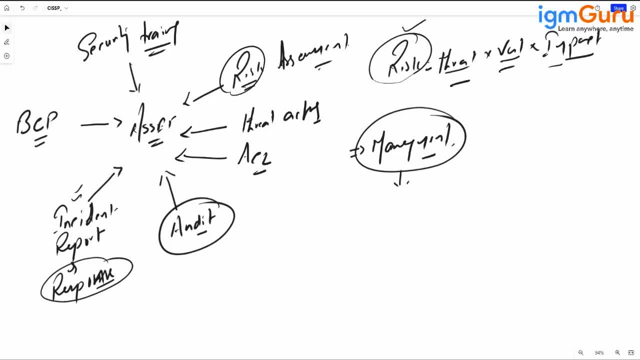 to this, different person and different country might be having different roles. for the same, like in some country, you will see czo, chief information security officer. for the physical security normally will take care of by the cso chief security officer, right? so some some places you will see the technical manager, okay. 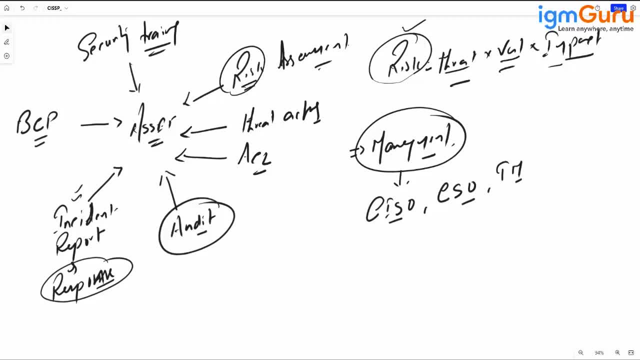 who will basically taking care of the security? remember, they are the responsible, but they will not do the implementation. implementation will be done by the administrators. so these are the role who is basically responsible for security of the organization and accountability belongs to whom? your management- ceo, cto, cto, chief technical technological officer. so they will be the. 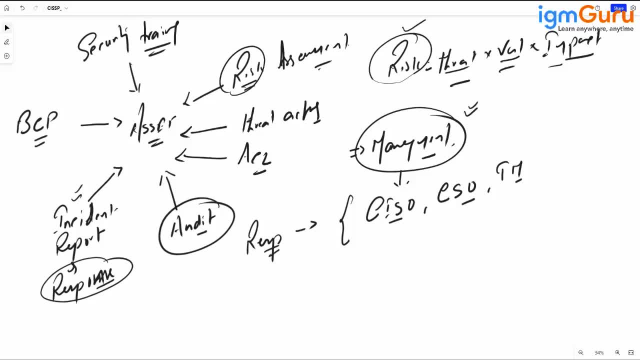 accountable person. so if they also commander disaster management team? no, no see, disaster management team is also one of the security capability which we have to do for, and normally that is the responsibility of the chief security officer: physical security. but again, it totally depends on what kind of disaster. it is right, logical disaster. 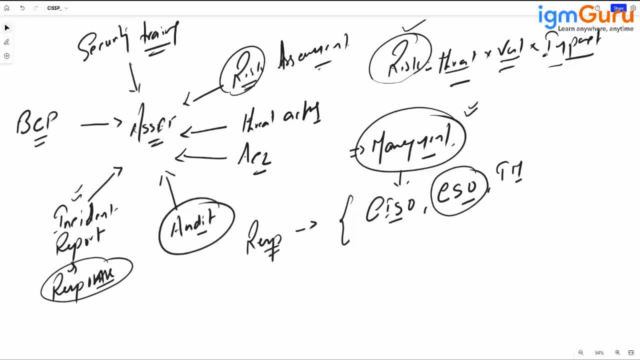 physical disaster. but at the end of the day, remember, when it comes to disaster, everyone is going to take care of that. but, yes, some role is responsible based on what they are managing, like chief security officer will take care of the physical security and czo will take care of the logical security of the. 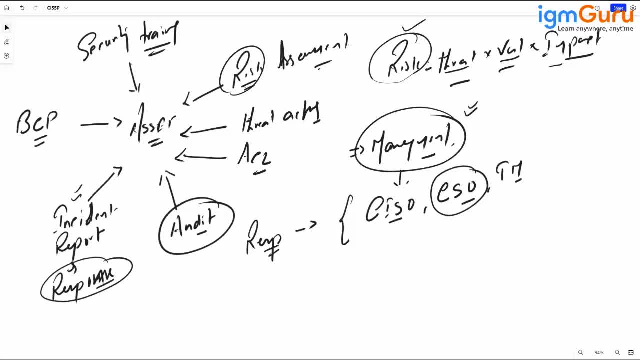 organization right such way. and one important thing another apart from that, that when we implement the control, there are two type of control. normally we have technical control and non-technical control. so in case of technical control, definitely the firewall, anti-virus, ips- these are the solutions we are implementing- and non-technical control, like policies. 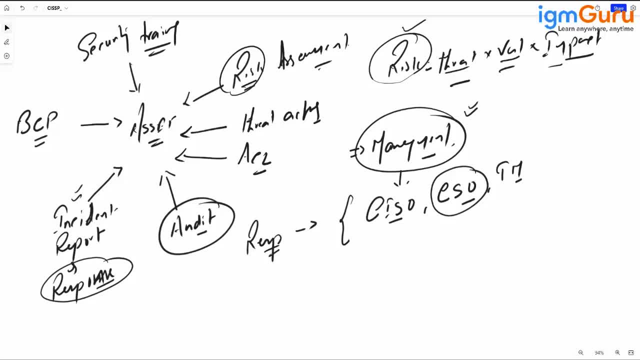 right, the standard guideline. so these are called the non-technical control. one such example is the separation of duty. one sensitive task cannot be done by a single person right, like, suppose, accounts. so normally one user will prepare the check, another user will will audit that check and third user might. 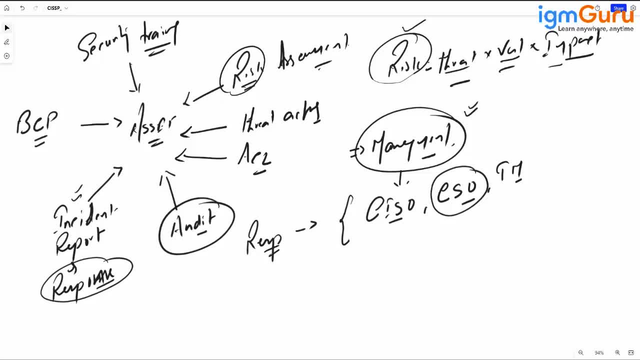 be hand over the check to the vendor. so this is called the separation duty, where we are ensuring that no, any single person is doing the sensitive task. if they are doing, the chances of fraud and fraud and fraud is not really going to be very much used or higher right. one important thing: 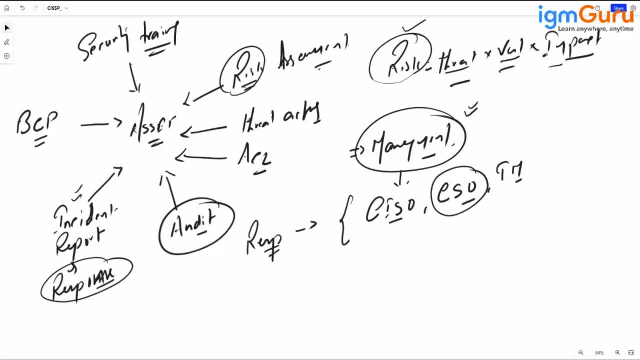 which we have to understand, that every organization have to ensure that they are taking the necessary care of the organization. so this is called the due care right. see, as a, as a technical manager or as a caesar, i have to ensure that i am doing my duke. i have a certain duty. 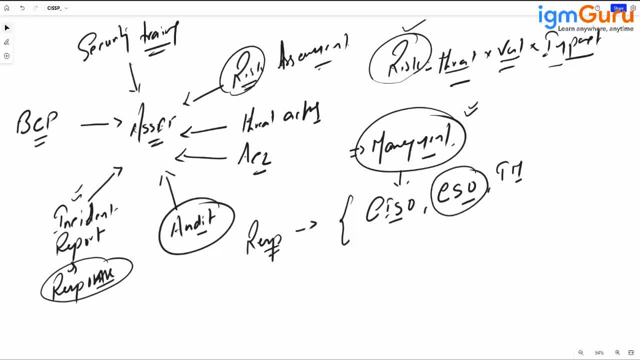 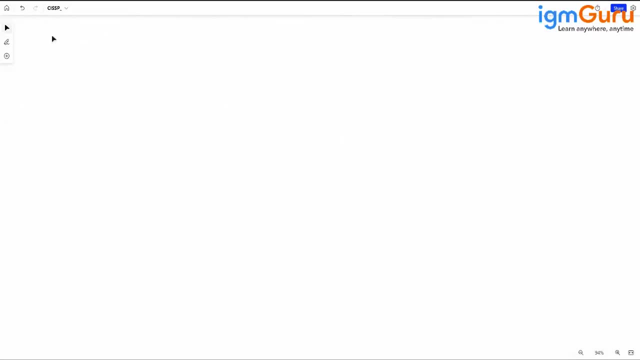 have to ensure my organization resources are protected right. so i have to ensure that i'm performing the necessary due care to protect the interest of the organization right by implementing the necessary security control right. so what we had understood so far- that what is asset and what is risk- now remember, whenever there is a risk, there are different type of control. you will be. 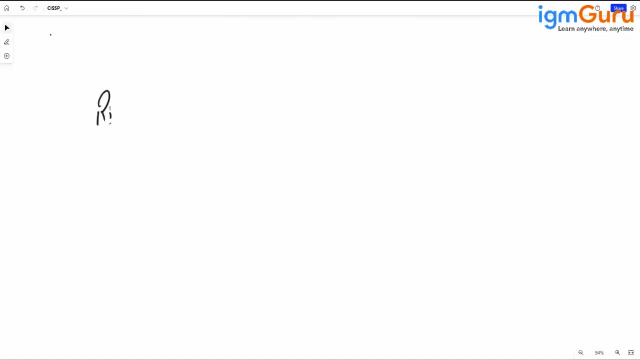 implementing right to manage the risk, you may have to implement different set of control. one such one such control is called as technical control right. so technical control means a control which is going to tackle the logical data issue. technical control could be a software. it could be a hardware right like firewall. so as an example we can take is the firewall. 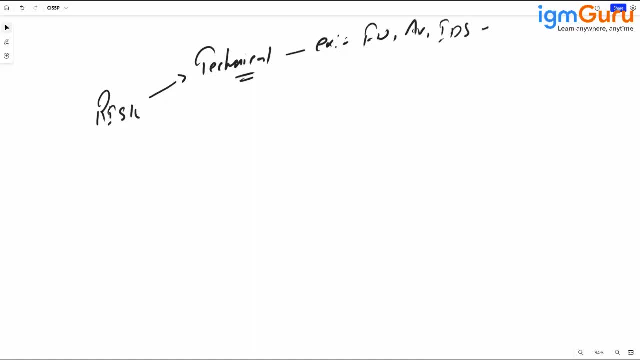 and antivirus ideas, right, etc. there's lots of other solutions available in the market, but these are the technical control. who will take care of the technical aspects of the data? another control we have is called the operational control right. so control that depends on a person for the implementation is called the operational control. 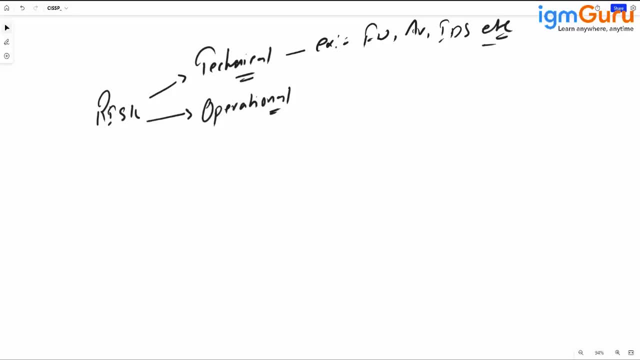 right. so simply, we can say: there are lots of activity within an organization. we do to ensure that all tasks are completed on time, right? so operational control will ensure that certain resources are protected in their own way, right. and similarly, we have the managerial controllers controls that give oversight of the system. how do we manage a system when there is certain 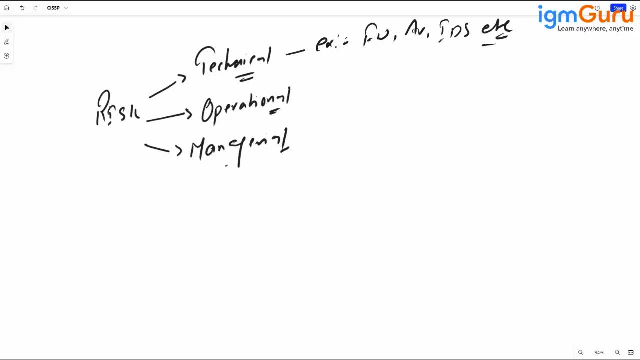 guideline in the standard available and we have to ensure that we are following that. so managerial control will take care of that particular thing. okay, all, we will take care with the�m examples in the future, but for now, yes, these are the different sort of control you may. 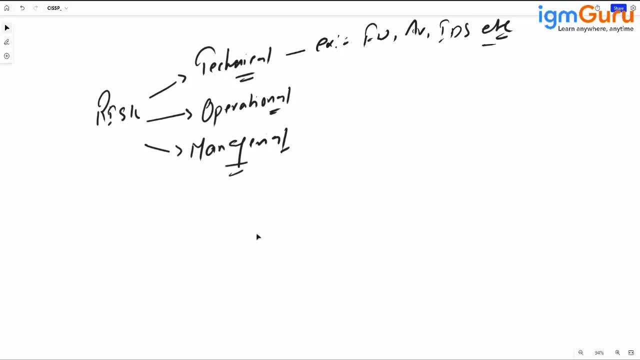 be implementing, but whenever we need to implement these control, remember, every control is having their own action. okay, yes, like some, some control is having detective action. detective means you are implementing a control through which you can detect the intrusion attempt. okay, okay, so this is called as the detective control. 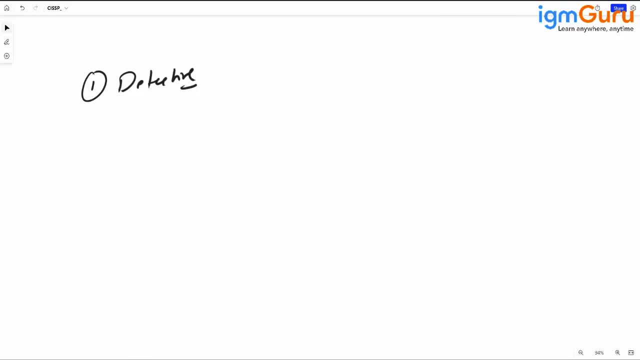 getting a point. that first one is detective. detective means we are going to detect the issue. okay, kapta, are you there? yes, yes, i'm here, i was, i haven't got. yes, and another control could be preventive. preventive means we are going to prevent the issue. let's suppose i am implementing. 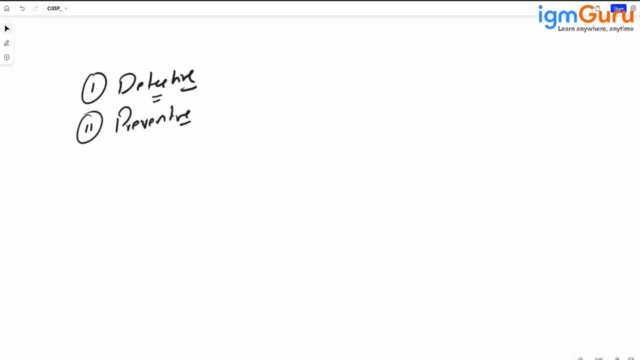 a door, door with lock. okay, yes, it will help you to prevent the intrusion coming to your house. so that is called preventive control. right, another control is going to be the corrective control through so you can correct the issue. let's suppose i have a backup for my system, so if there is any data loss, 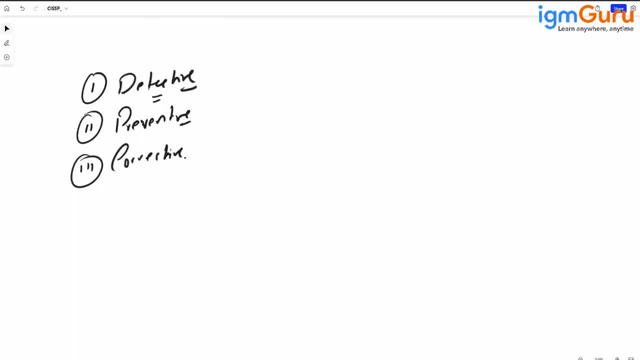 i can correct the situation right. so these are the major control type we have there, right, but definitely we have other controls as well, like we can also have the deterrent control. so you must have seen any negotiating decision okay. so any, whatever scenario are happening or a lot of things. 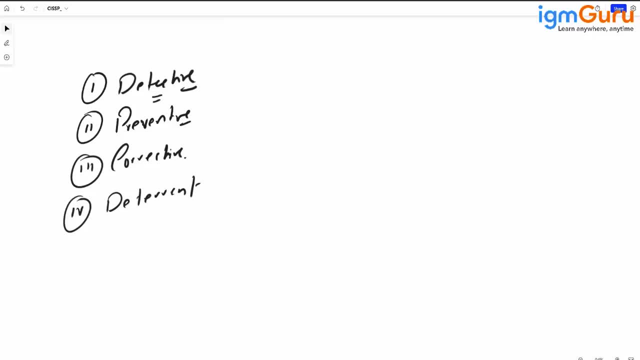 happening. okay, but i want to know, i want to know about some scam part which i have seen. is there research in other departments? yeah, if there is another, a case como, such as if there is another scam or you know before, which are listed on the internet sometime you are under the cctv的时候. 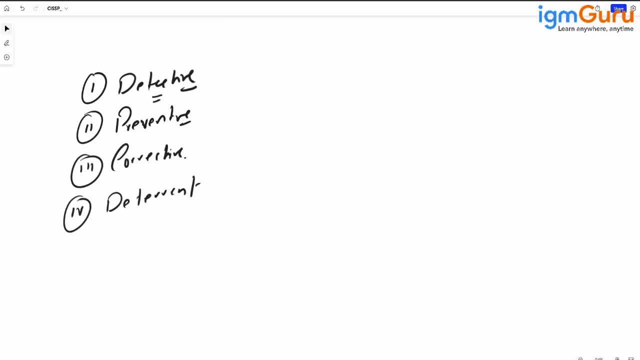 d часто에 эти �KAZ. you can't predict which will be the mac書. this aing pap tree is known in aoga right. so detent control is just to deter the user. it is not definitely going to stop the user or. 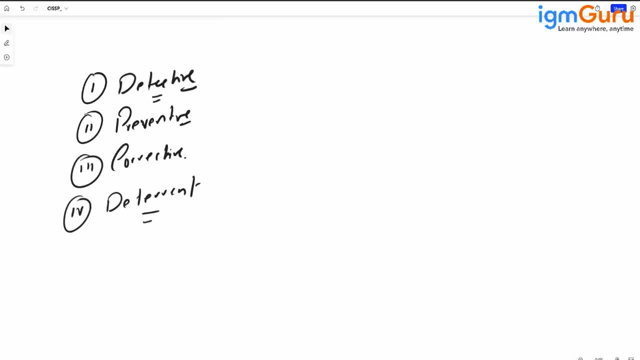 stop the attacker, but at least it is going to make them attentive. yes, okay, i'll give. give them a heads up. that, correct, we are being watched right. another control is compensative control. so compensative control, to understand this, let's take an example here. let's suppose we have a server. 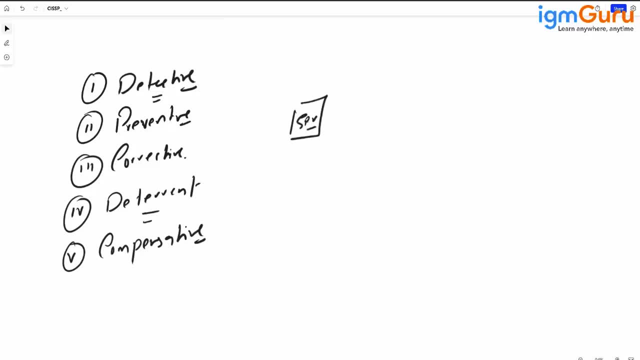 this server is a web server right now. normally to protect the web server we keep firewall in front of the server. so whenever any user is making requests, first request to come to the firewall, firewall will do the filtering and then only it will reach to the server. but firewall can filter the traffic based on a specific address, like ip address and port number. 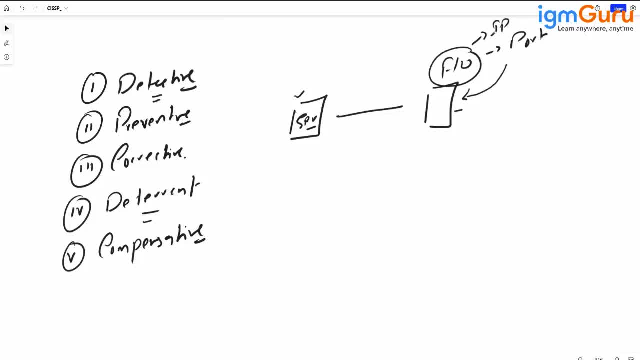 right, mm-hmm. but let's suppose attacker is doing some application based attack. it will not prevent. so in such case we have to implement a compensative control. compensative control could be a web web application firewall. so if firewall is not able to prevent, then web will prevent that attack. 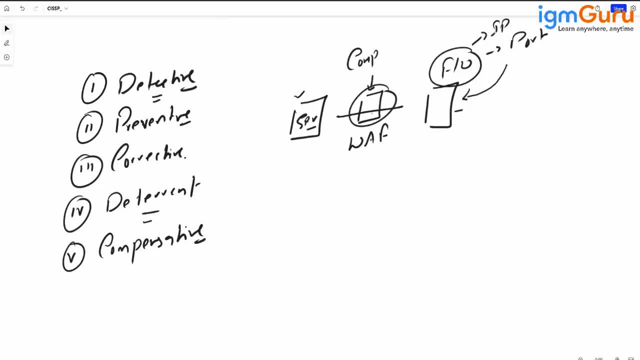 it means compensative control is compensating the issue which the firewall cannot resolve. my primary firewall cannot resolve. so in such is it like a second layer of protection. we can call a second layer of protection, yes, you can tell, but that second layer is basically tackling the weakness of primary control. 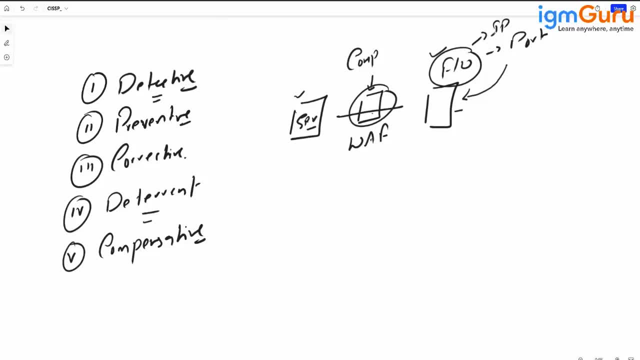 right. it's only not only stopping the Imagination that we can called as theê the trick, it also trying to figure out what went wrong with the first facet of the correct. you can see, yeah, fix my Kenny of control it. They do that. 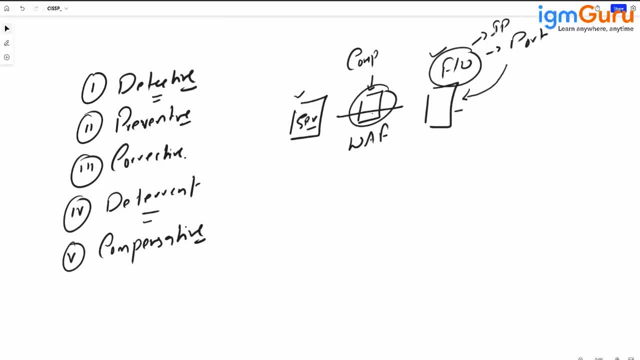 So this is on other control, for is a little bit incitsu from the default. Yeah, for the lifetime, we have to atualize the agent you will implement right, but all in all, these, all are the different control, which control action which will help you to protect now what we had talked about, the risk, we had talked about the 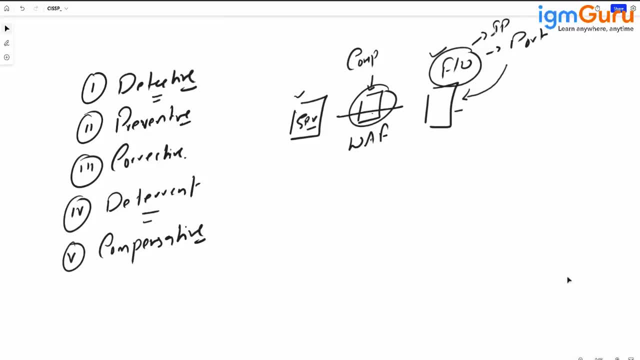 control, right, but when you go and implement these all controls together, as i told, that is going to be quite messy. when you have to start first, right, and that's the reason. let me go through all this once again, please. yeah, yeah, sure, thank you. so, as i told, 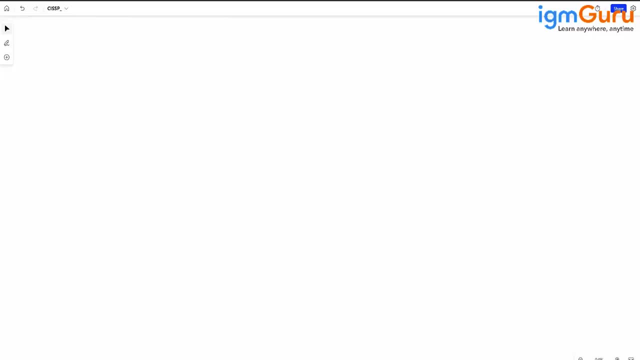 that i will come back. so, as i told that it, when you are going to implement, that is going to be quite messy, right? so in such case, what we do, we take a support of cyber security frameworks, right? so frameworks will basically going to provide you the structure and guideline, and 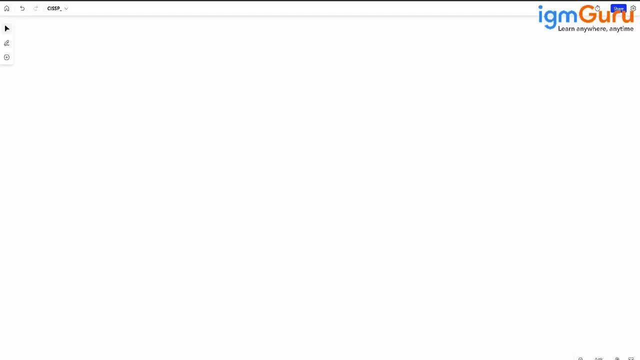 then it will tell you: hey, what are the controls you have to implement, right? so if i get a guideline that these are the controls which will help me to improve the security, then it will be good. in such case, i know that what are the works i have to perform, right? so there are multiple. 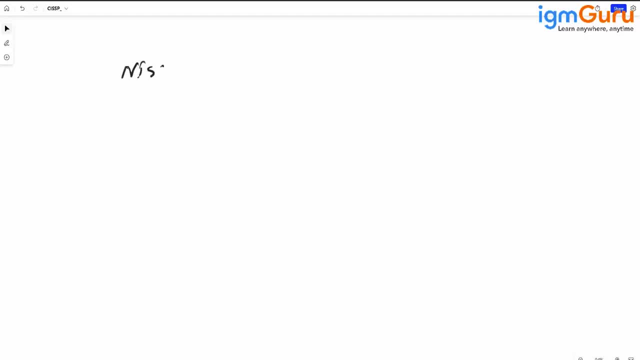 frameworks we have around us, like one of the framework is available from nest cyber security framework of nest, national institute of standard technology, cyber security framework. so nest has given cyber security framework, csf. nest has given risk management framework which is actually telling you how to detect the risk and how to respond to the risk. 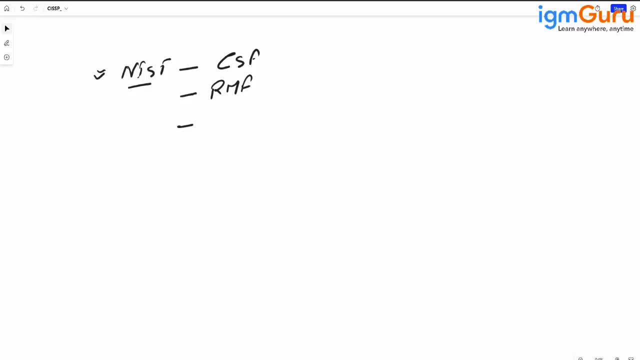 one of the major control we implement to manage the risk is encryption. in the future session we'll talk about the encryption, but for now, understand, encryption is a converting your plain text information into cyber text. okay to do the encryption. we have a certain standard also available that is called fips- federal information processing system, or processing. 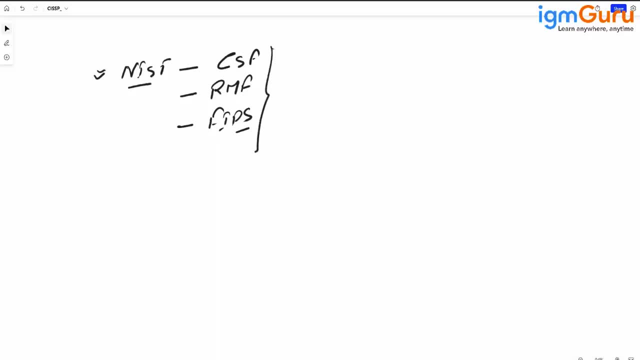 standard and apart from that, lots of special publication, normally nest publishes, which will help you to guide- let's suppose you have to do the risk assessment. so for the risk assessment they had done, given nest 830 is one of the special publication, you can see a white paper published by the nest. similarly, for the risk management framework. 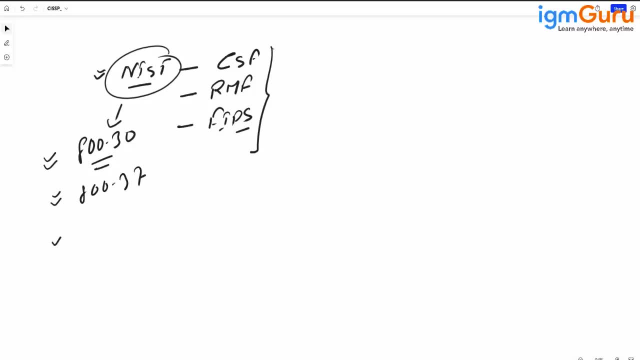 they had published 837. right for the control implementation, they had published 853. for the data classification, they had published 860. so there are lots of special publication they had already published which will help you to guide. let's suppose you have to do the risk assessment. 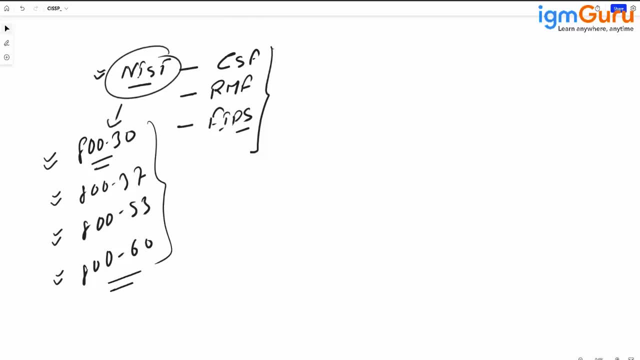 which will help you to guide how to implement the cyber security in your organization. it means you don't have to work very hard, but, yes, you have to go through the documentations which will help you to understand how to move forward. but nest is not the only person which 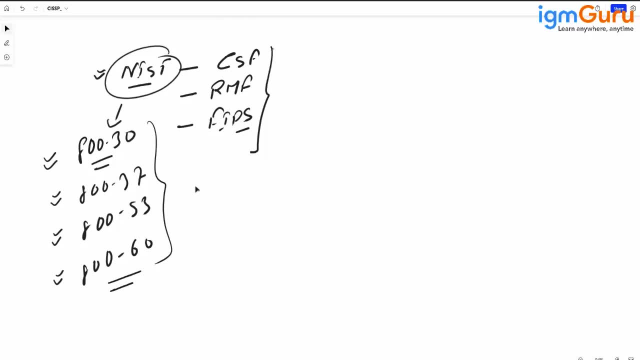 is there in this market, right apart from the nest. apart from the nest, we have other vendors as well, like one of the most popular vendor in this uh places. i don't know. i don't know if you are familiar with it, but i don't know if you are familiar with it. but i don't know if you are familiar with it, but i don't know. 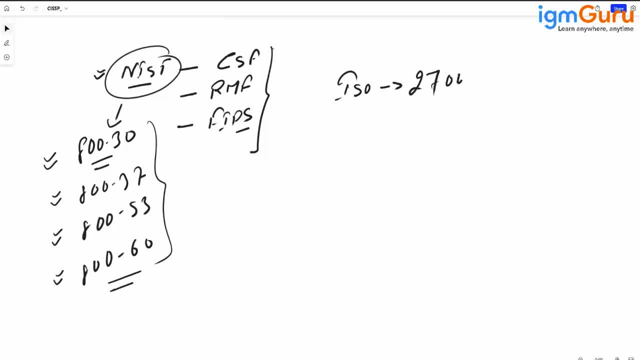 if there are anyister game you can download it and get the complete старthar and ISO is having their iso 27000 different standards. like one of the gold standard for the information and technology is 27001 ISO 27001 right, which is called as information. 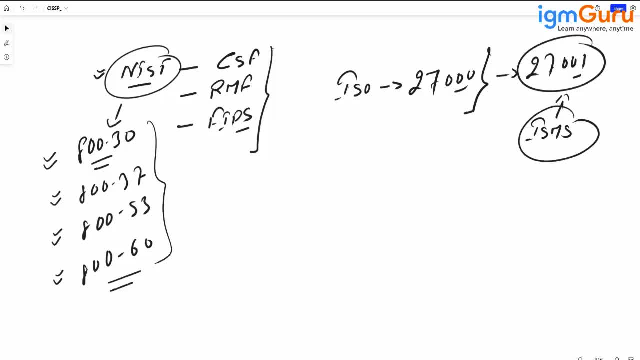 security management system standard, ISMS standard. so whenever you have, you are managing information system. to secure that information system, the standard which we follow is a ISO 27000, is a iso 27001 right. similarly, if i'm going on cloud for the cloud, we have csa standard. 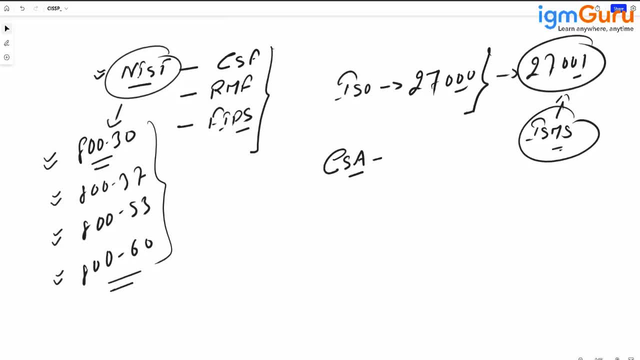 cloud security alliance. enterprise cloud control metrics standard ccm right. uh, if, if i need to do audit, for the audit we have a certain guideline also available. like normally, the service based organization will conduct the audit and for that there is also standard defined which is called the service organization control, and under that they have 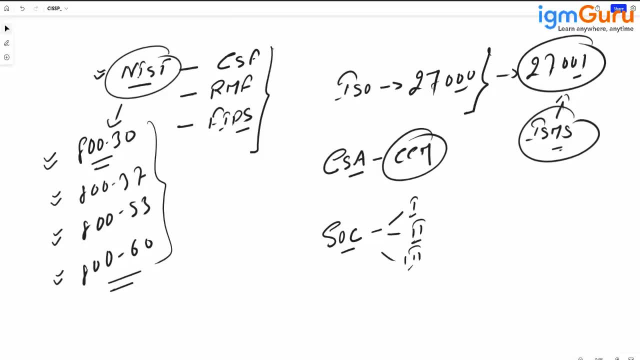 sock one, sock two and sock three. right again. right now it is not needed to be uh to know about all these things, but for now you have to understand that whatever we do, there is a certain standard and frameworks already available in the market. it means we don't need to work very hard. but yes, we. 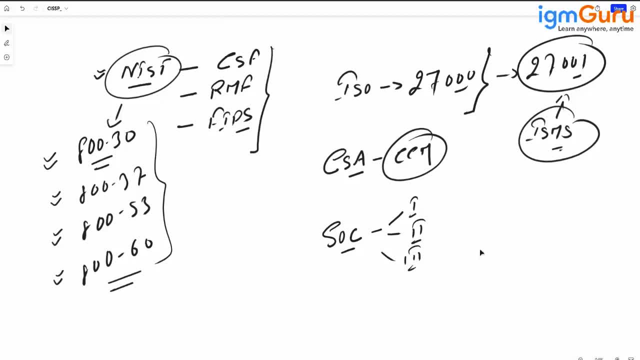 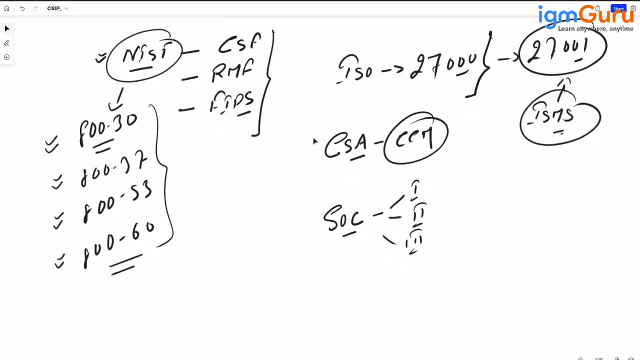 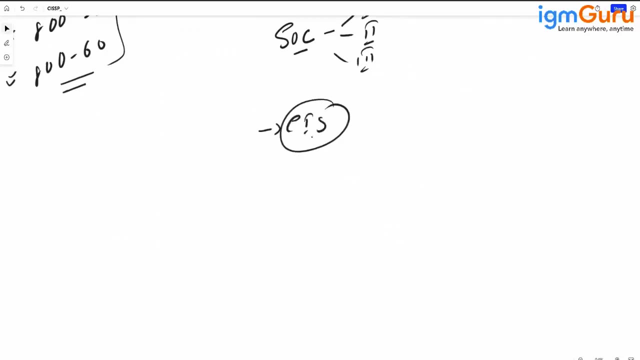 have to understand these documentations, go through with the documentation and then understand how to implement those documentation right. similarly, if i'm implementing control, then we also have the cis benchmark that is called center for internet security. so there are total of 20 cis controls available, which is actually telling. 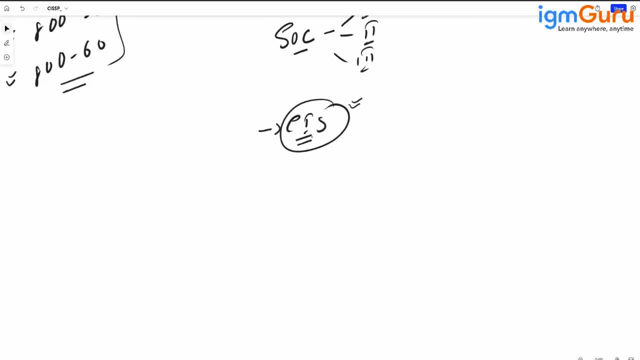 you? what are the controls you have to implement to secure the system right? if you're trying to secure your application, then we have a osp that is called open web application security project. so that is another standard available. so, as i told, whatever we do, there is a specific standards available from the different different vendors. but all it totally depends on the country. like us and canada normally follow the nist standard, so much okay. and if you go to the european market normally you will see the iso standard is so much followed there. but again it is also totally depends on the interest of the organization and the kind. of customer we are managing, because sometimes the kind of customer is coming to you and they are asking you: hey, i require you and your organization to be certified from iso 27 000 standard. i will not deal with you if you don't have that certification available with you. so 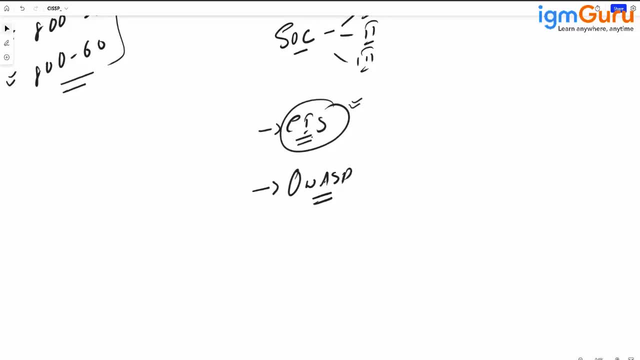 organization also certified themselves. they prove that, yes, we have all the necessary measures through which i can secure your data, and if they will not give you such kind of- uh, you know, trust this, then you may not able to go into business with them. okay, so that is the reason we have to. 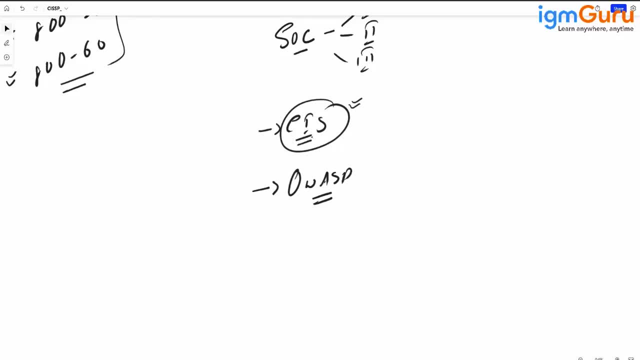 have all these standards getting implemented in the organization, sometime only for our benefit, and some time to prove our customer that, yes, we are doing all the necessary care, okay, okay. so at the end of the day, remember, it's a. it's a i mean from the information security side, it's the due diligence effort. 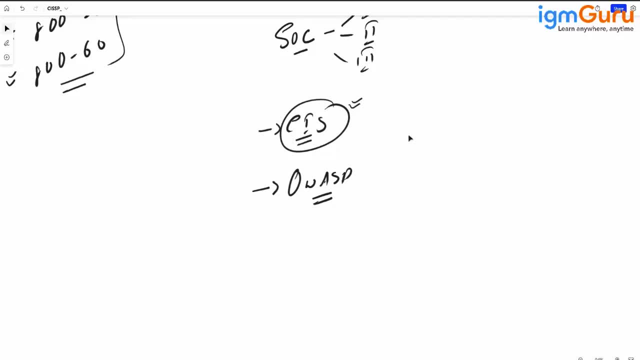 so due diligence, remember is, is an ongoing effort. ongoing effort means so today i had implemented the control. it doesn't mean that i'm now i'm safe. i have to continuously evaluate the effectiveness of the control and ensure that we are keep updating the controls and managing it properly. 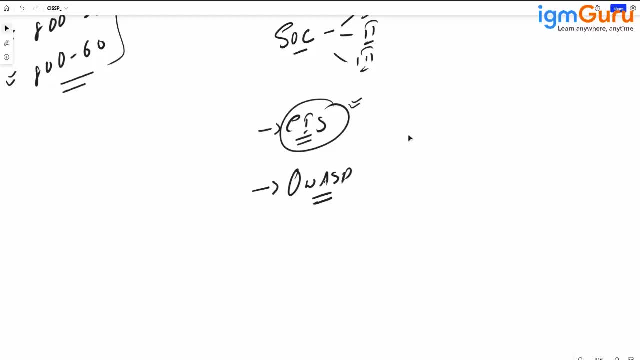 right, like selection of an antivirus after researching the market is one example of the due diligence. and after the implementation, continuously updating the antivirus is also what the due diligence only. so continuous update will never stop. correct, it will, it will always go on, but yes, after researching about the antivirus and then implementation of that antivirus. that 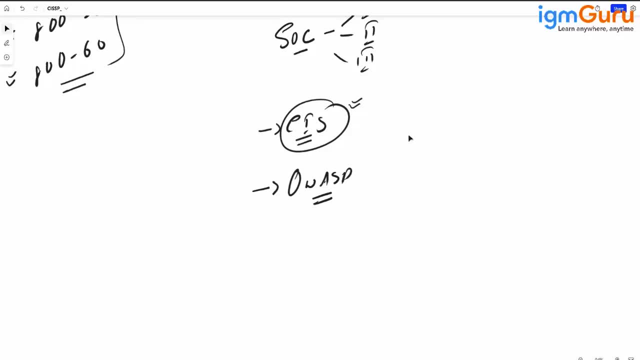 is called as due care. it means you are taking care of your resources. and then again the multiple methods which will help you to do that, multiple apps available, like when you are working for european market, so for european market. one of the critical regulation they have is gdpr- general data protection regulation- where we are ensuring that- if i'm 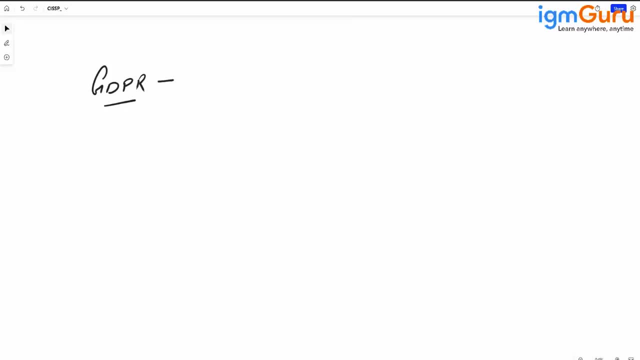 storing any information about the european customer, then their data is called as pii. it's called personal identifiable information: their name, their, their contact name, their- you know their- social security number- right, so these are basically falls under the pii. so we have to ensure that we are protecting.